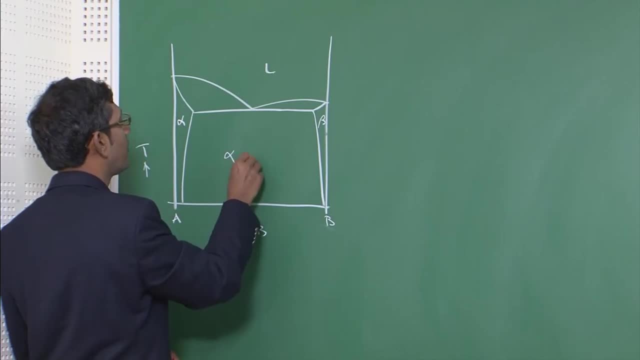 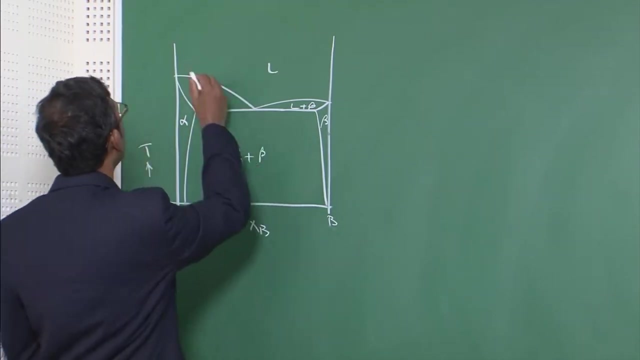 end and B end respectively, and this is alpha plus beta and this is alpha plus liquid. this is liquid plus beta. So there are three two-phase fields and three single-phase fields. So we are going to draw the free energy composition diagram for this generalized eutectic phase. 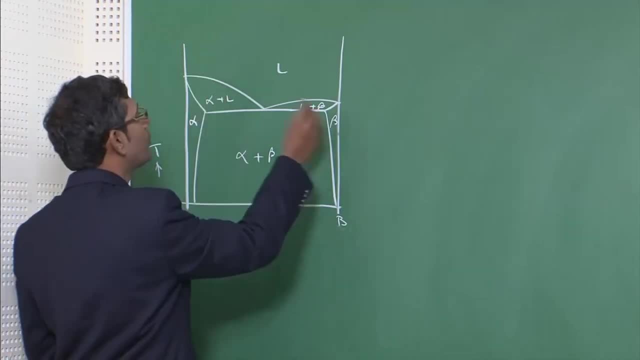 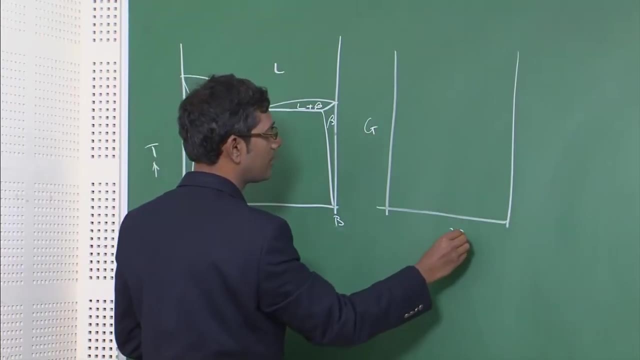 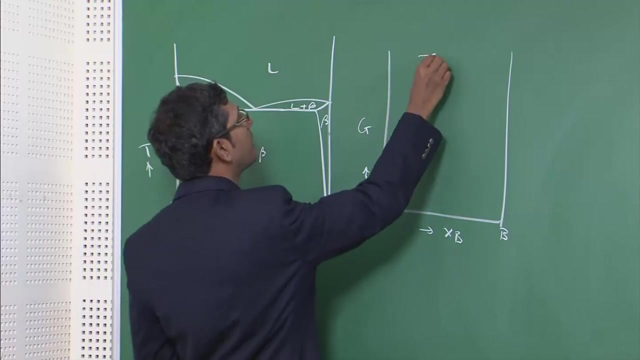 diagram. You can draw it others very easily and as I show you, the free energy composition diagrams will be like this: This is G versus XB curve of the phases present here at different temperatures. So temperatures which we will select are like this: We will select temperature. 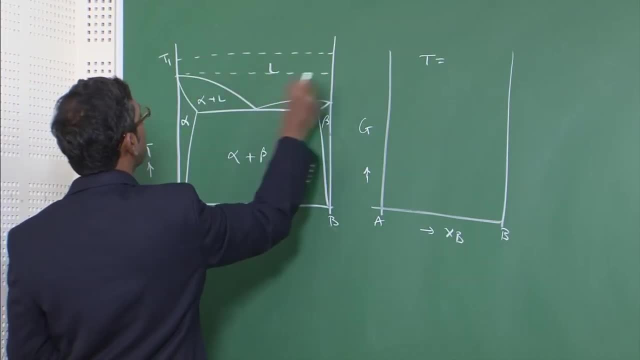 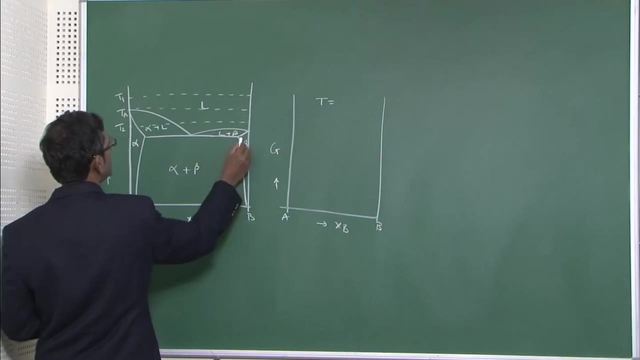 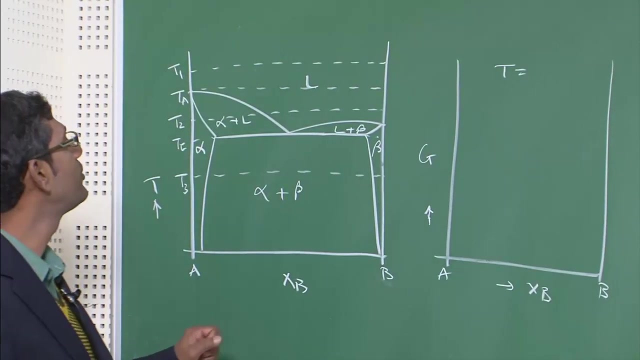 like T1, and this is TA, and then we will select the temperature here: T2.. This is TE, the eutectic temperature, And we will select the temperature at T3.. These are our generalized temperatures and basically the way I have selected temperature is that this will provide you different kinds. 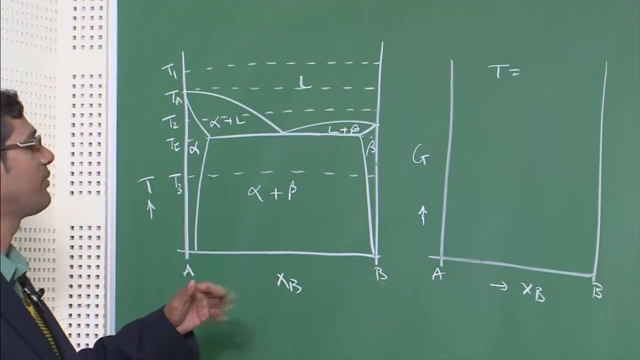 of possibilities exist when you draw the free energy composition diagram. So what I mean to say is that, at these temperatures, I am going to draw the free energy composition diagram and show you that. So what are these free energy composition diagram? Let us restate. 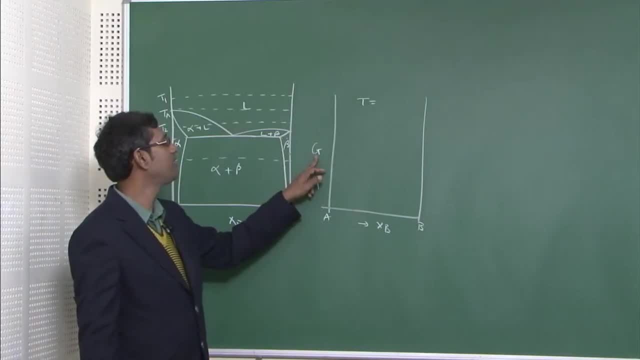 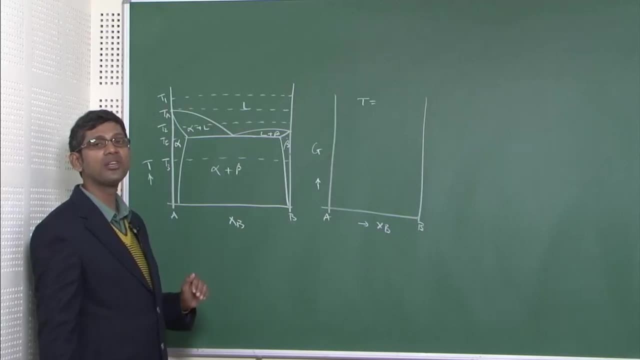 again, These are actually free energy means. give free energy versus composition diagram at different temperatures to show the relative dispositions of different free energy curves. What is that Suppose? at temperature T1, I know that the only phase table is the liquid, all the composition from starting from pure A to pure B. Now to show that we need to 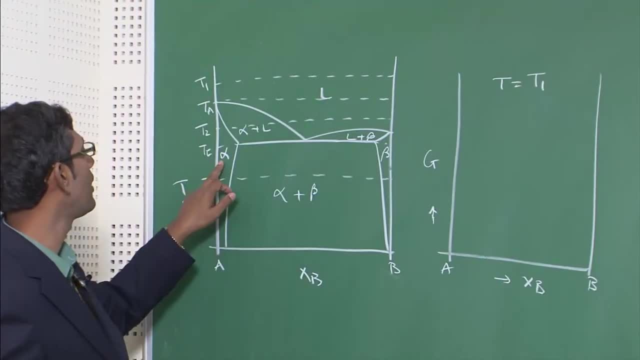 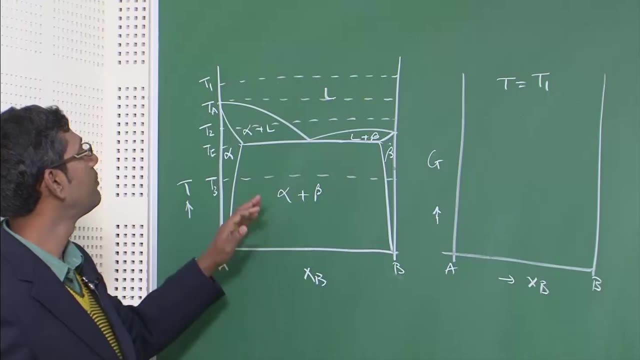 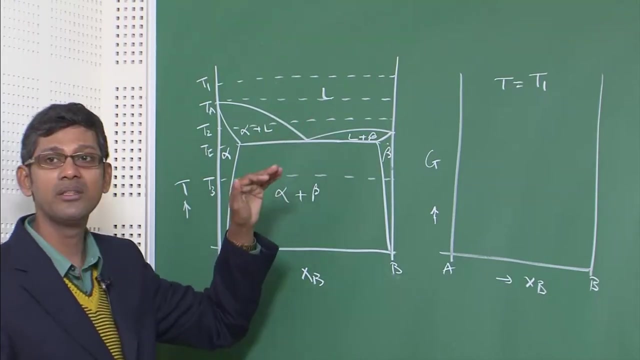 draw the free energy composition diagram of liquid phase, solid alpha phase and solid beta phase. And it is very clear, and you probably have understood, that because liquid is stable, only liquid is stable at T1 temperature, so the free energy of the liquid will be minimum. 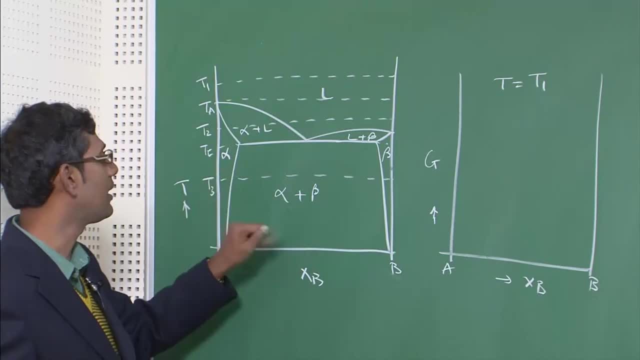 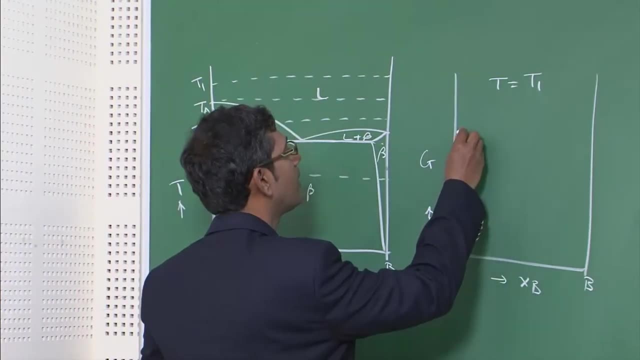 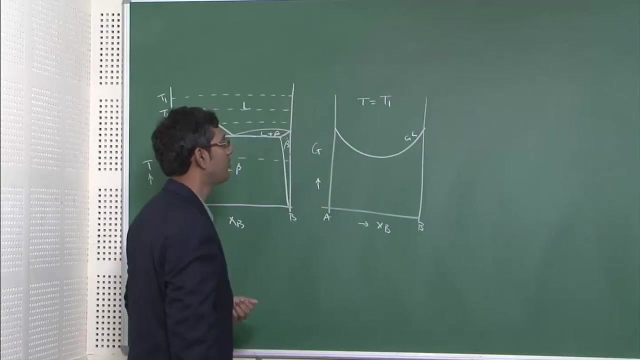 The free energy of other two solid, alpha and beta, will be above that. So let us draw that. So I will draw free energy of this liquid first, Okay, Okay, All right. So which is by solid line, this is PNG of the liquid and I will draw PNG of the 2 solid. 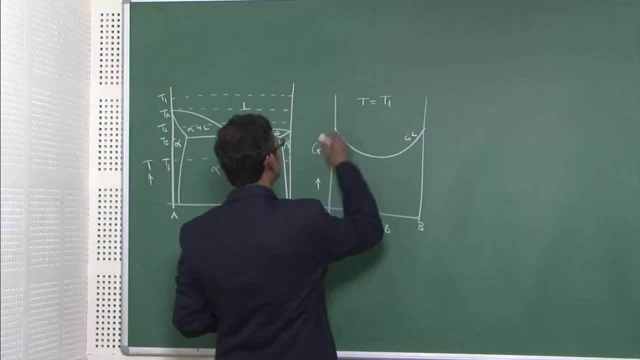 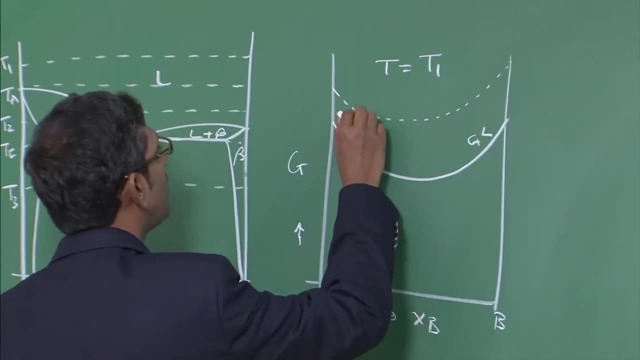 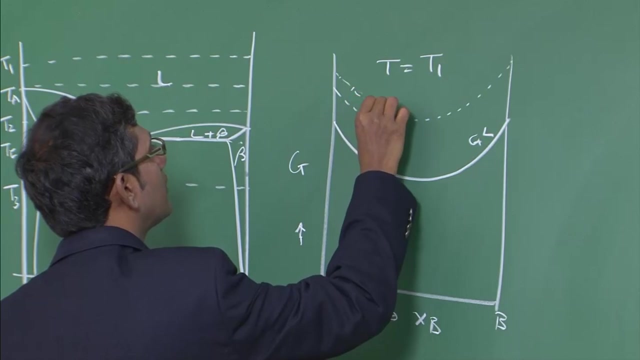 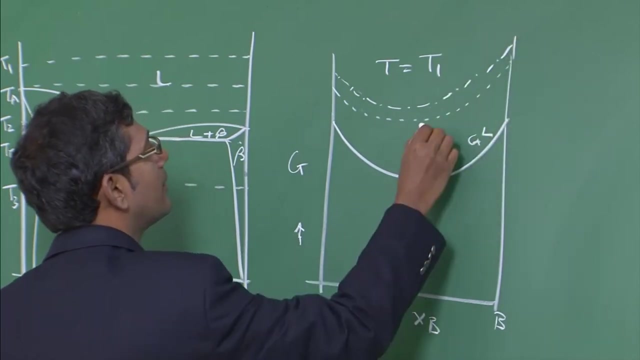 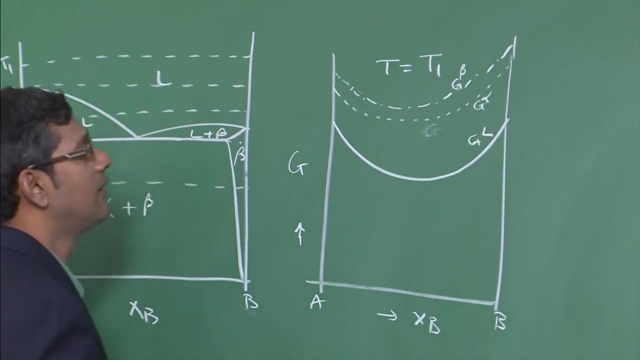 phases: alpha and beta. let me draw like this: So I will draw by alpha1 by dotted line and I will draw beta1. also will be by different dotted line. okay, So this is G, this is G alpha and this is G beta. right? 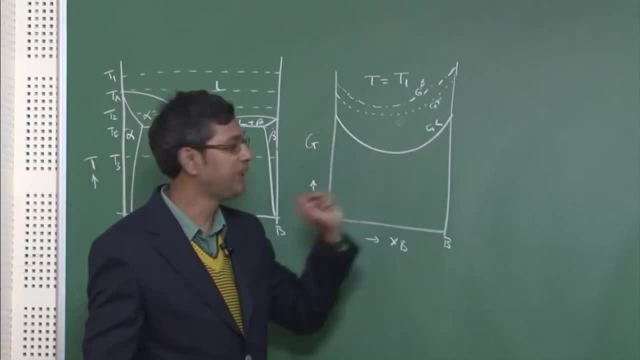 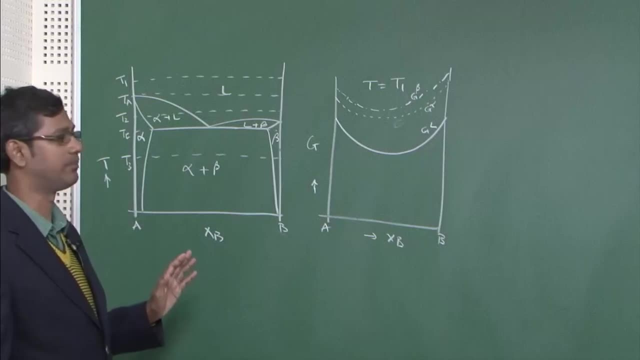 So you can clearly see the liquid phase is minimum at all. composition from pure A to pure B. Shape of the pheniagrid curve remains same. that is inverse parabolic. Okay, It does not change. and I told you why it should not change, because this is a depends on entropy. 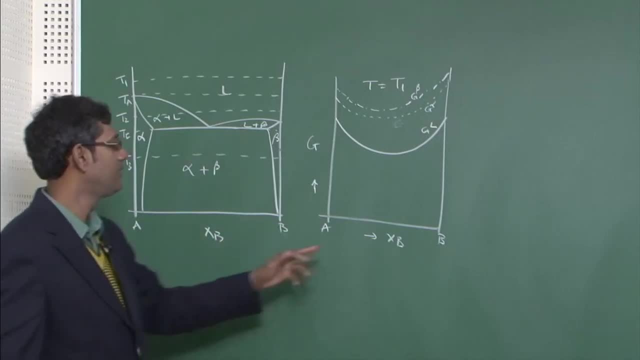 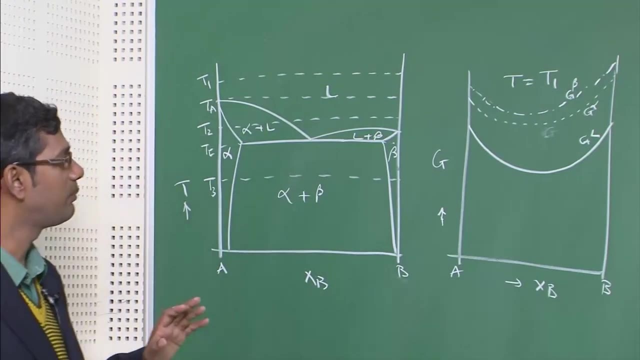 and enthalpy, and both of them are functions of the XB square, So that is why they look like a parabola. So that is very clear. So that, but the message is that whenever you are drawing pheniagric compression diagram, 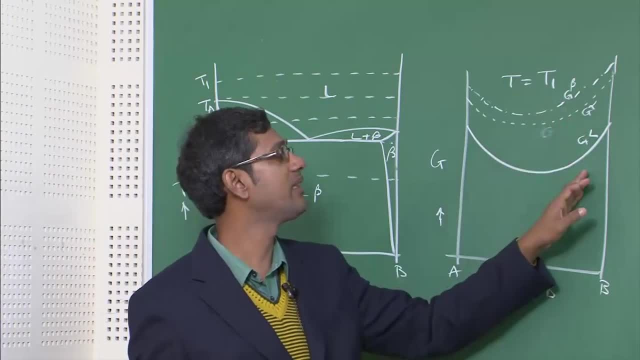 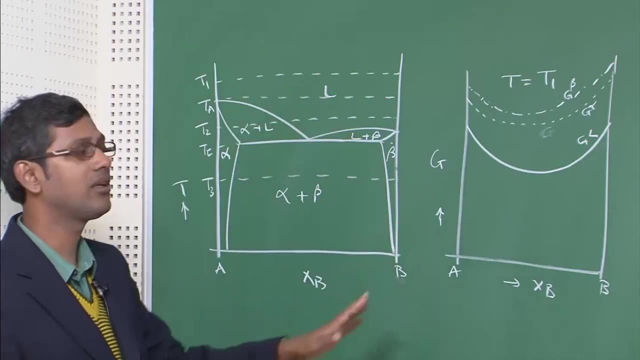 in a particular phase diagram, you need to draw the pheniagric diagrams for all the phases. Whether at a temperature- T1,, only liquid space is available. Liquid space is stable or not, that does not matter. What is important is to show you the relative positions of the pheniagric curves. 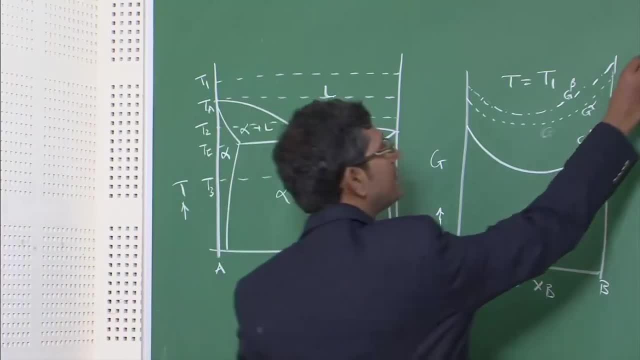 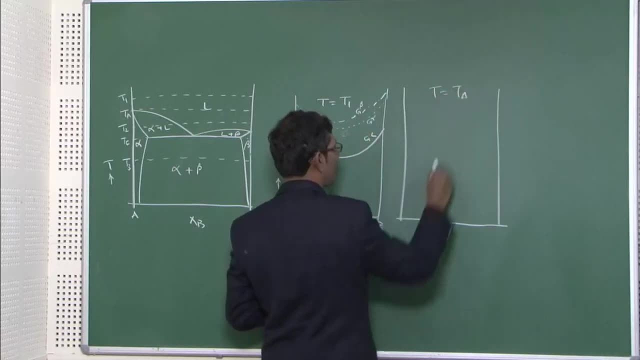 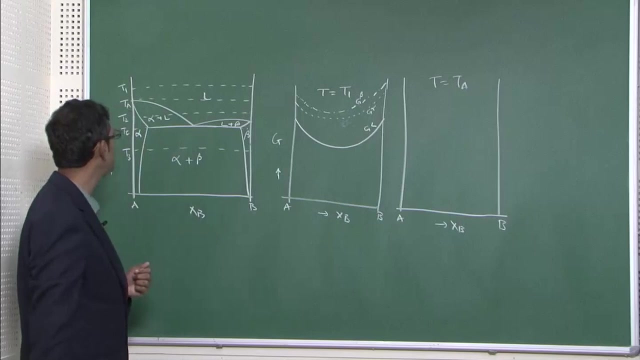 That is very important. So let us now do it at TA. So at TA, as you can see, I have already done it for your isomorphous system At TA. what is going to happen At TA, you can see here only at temperature: A temperature at A end it is going to be. 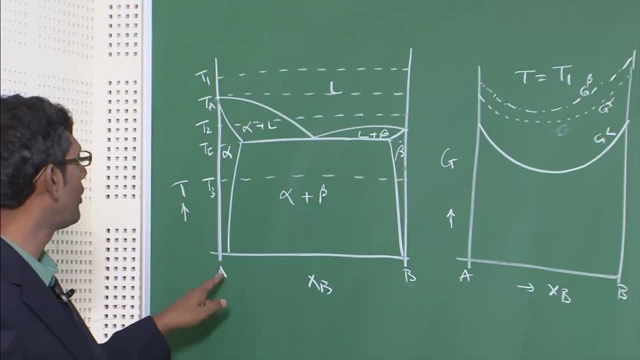 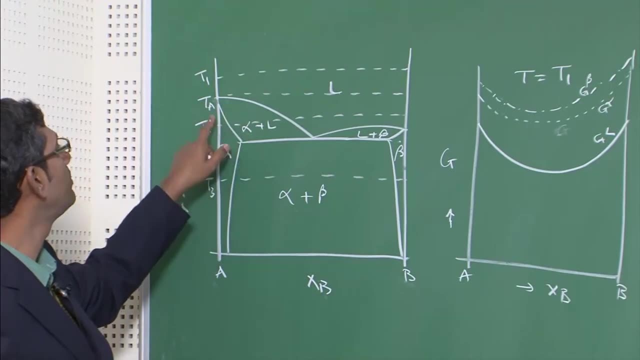 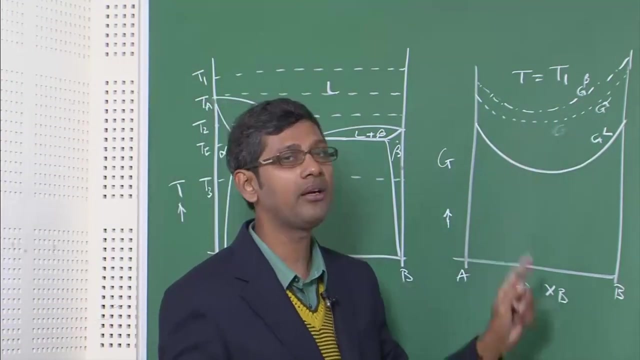 0. At A end, that is, compositions of XB equal to 0,. at the pure A end, the liquidus of alpha and liquid solidus of alpha meets. So that means what? The pheniagric curve of liquid and alpha will meet only at pure A end. 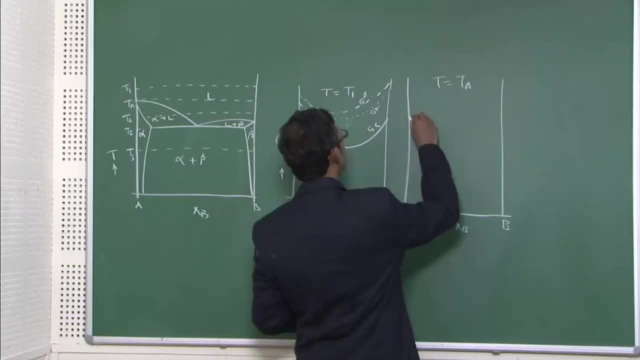 Others it will remain same. So again, I draw liquid. So, as I told you only at A end, liquid, Liquidus of alpha and liquid will sorry, alpha, liquid will touch. that is what you see here. It is touch. 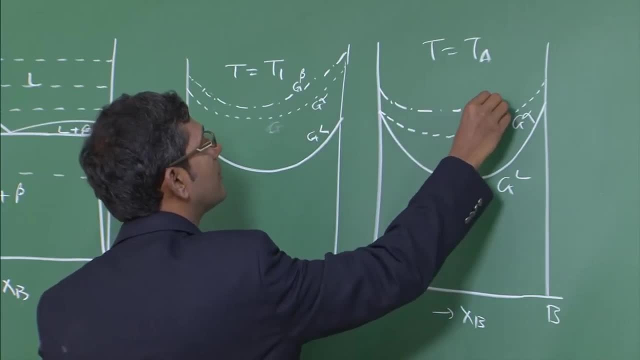 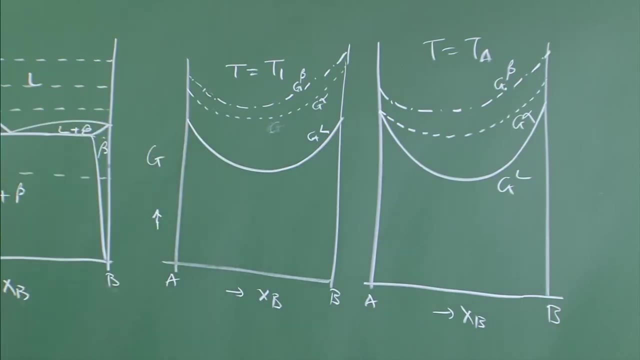 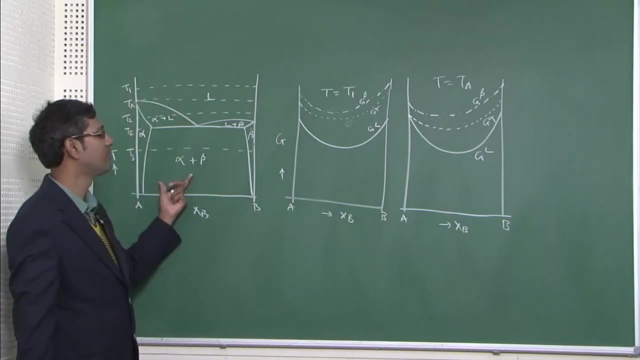 And beta will remain higher. okay, That is how it will look like, very simple. And these diagrams actually are shown, or obtained from this. By looking at this diagram? Okay, By looking at the phase diagram. that is why it is very easy to understand. 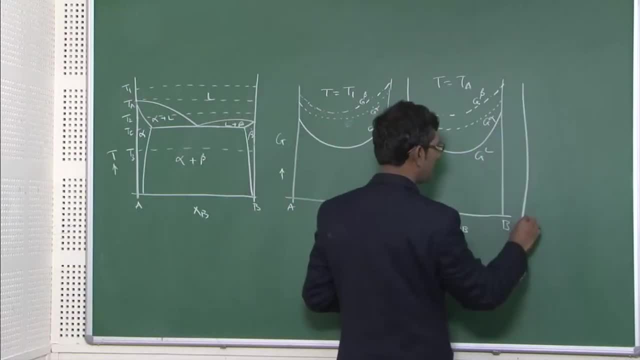 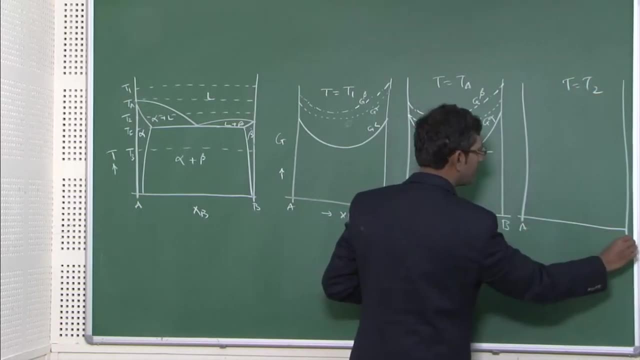 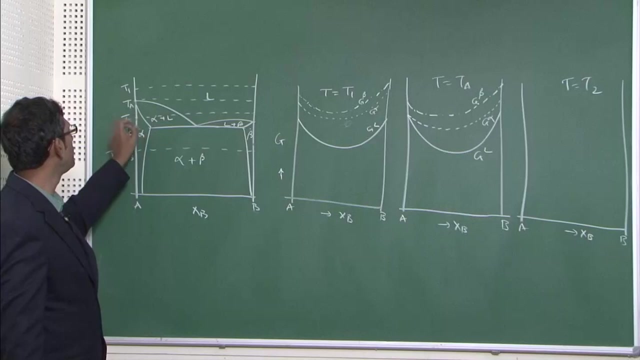 Now I will do it at temperature T2, which is also very easy. Temperature equal to T2, this is A, this is B, XB. So at T2, you can see, this is the most complex situations. At T2, there is a composition range in which pure alpha is stable. 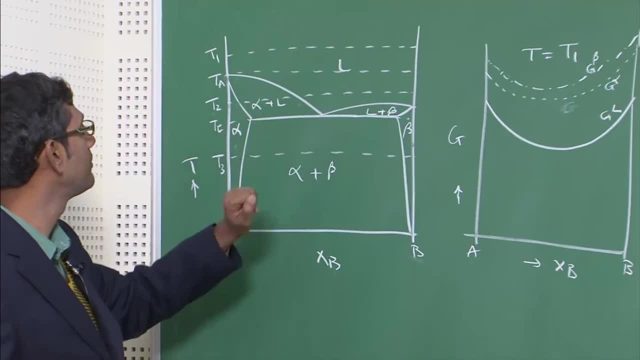 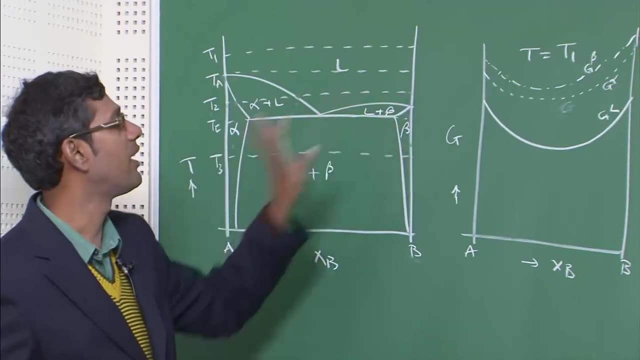 There is a composition range with alpha, and liquid is stable, And there is a composition range in which liquid is stable. So there are three: one, two and three domains. One is pure alpha, alpha plus liquid and liquid. So how to do that? 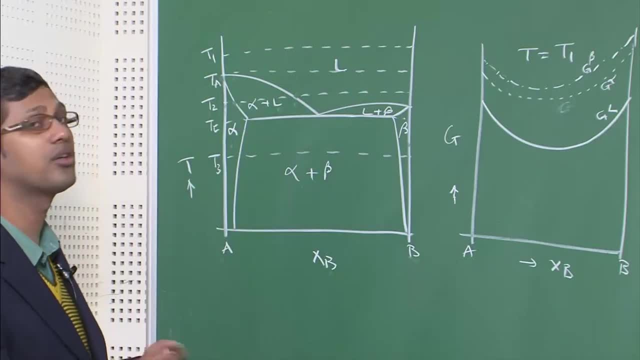 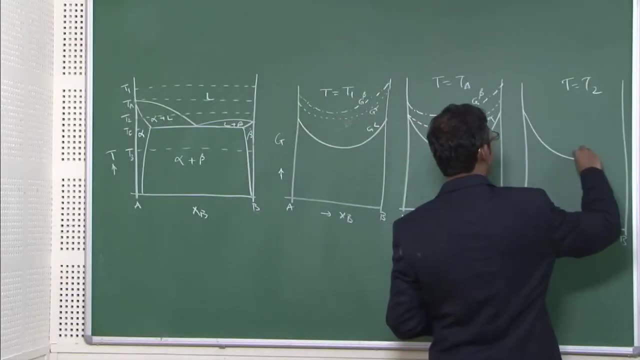 Whenever you have a two-phase field, I told you that pro-phiangic curves will cross over each other. So that means phiangic of alpha and liquid will cross over each other. How would I do it? Okay, First let me draw phiangic curve of the liquid. 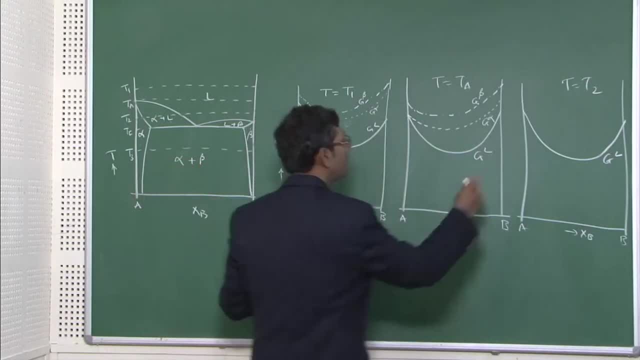 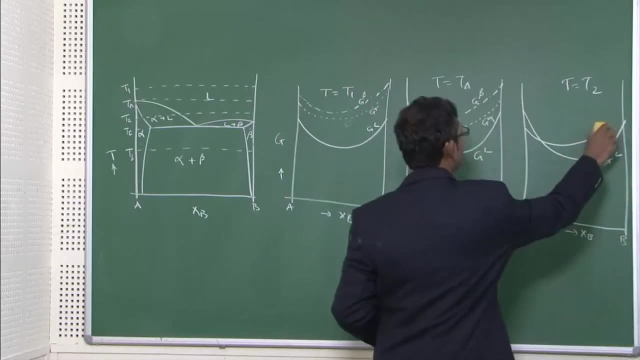 And alpha, obviously because alpha is stable. Okay, This is not the pure end, So alpha will be coming down. Sorry, This has to be drawn dotted line, otherwise you will be getting confused. Let us draw it. So this is G- alpha. 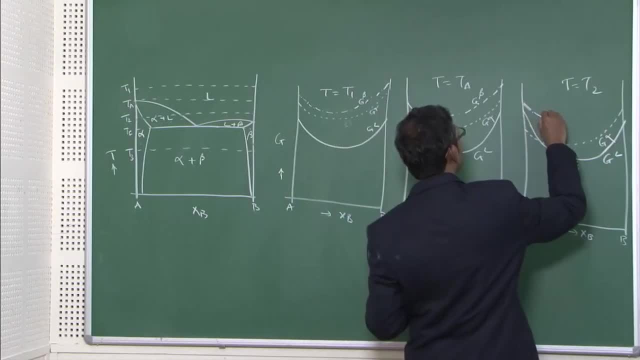 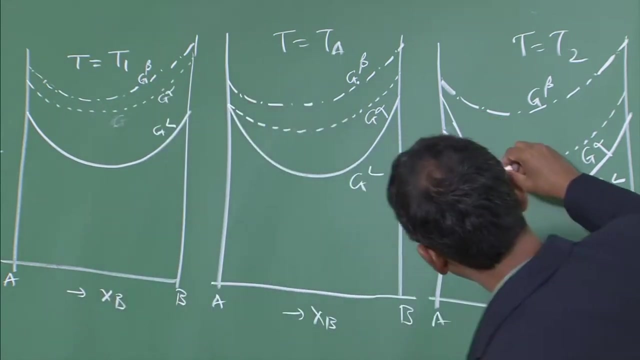 And beta is not stable at all. so beta will be coming much above. because beta is not present here, This is G beta. Okay, So when these two phiangia between alpha and liquid are crossing each other, the real stability will be obtained by drawing a common tangent between these two. 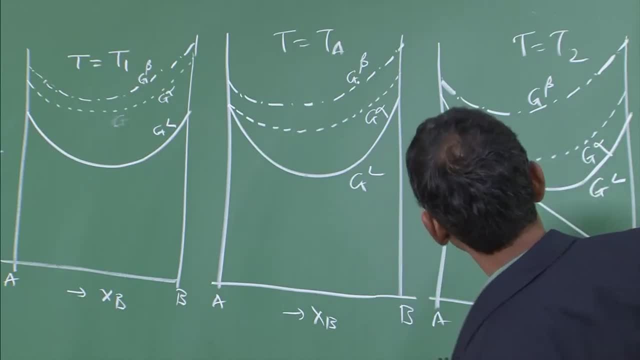 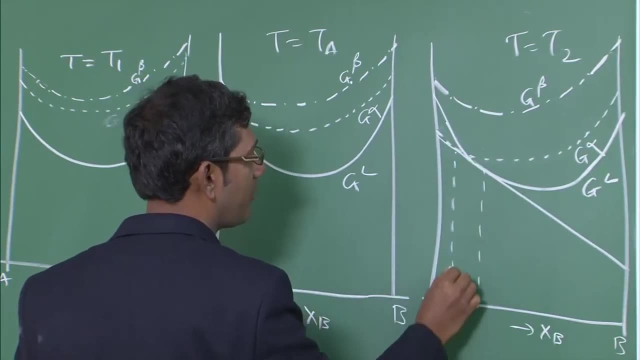 So let me just draw a common tangent like this. So if I draw a common tangent, it will cross or it will cut the liquid curve here and the alpha curve there. Okay, So that clearly tells me very simply that this is the stability zone of alpha. 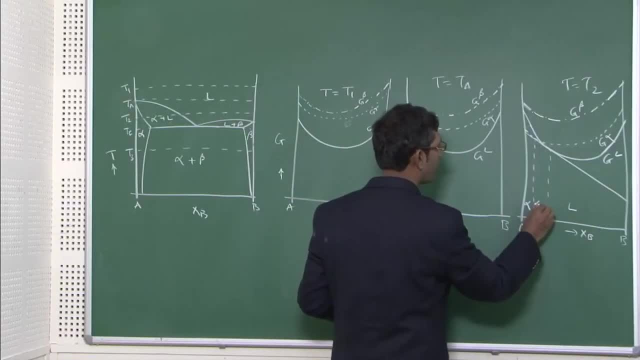 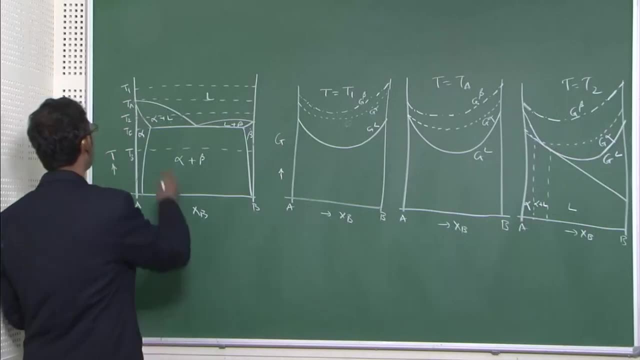 This is stability zone of liquid. Okay, This is stability zone of alpha plus liquid. That is what you see in the phase diagram. Alpha is stable here for the small composition zone. from here to there, from here to there, and then alpha plus liquid, and then liquid. 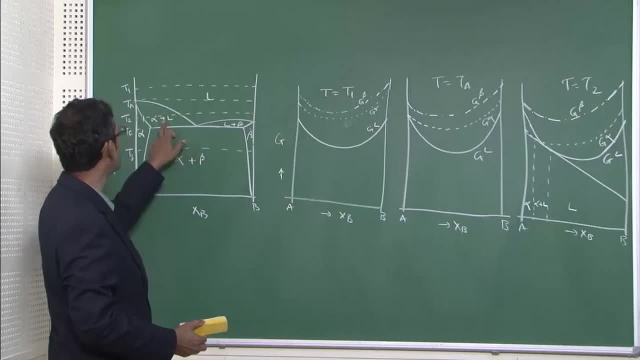 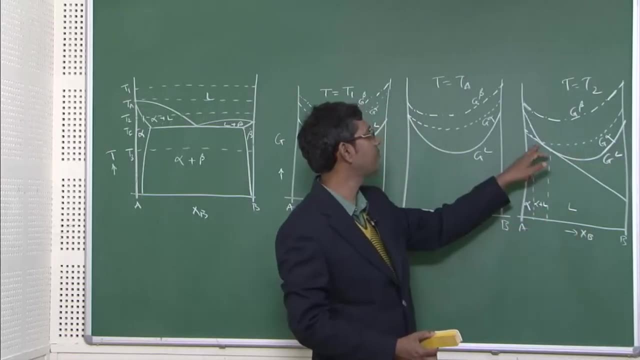 So one thing you understood: whenever you have a two-phase field and tie line at temperature T2 passing through the two-phase field, these two phiangia curves will cross over each other, and thus must be done. otherwise you cannot have the condition that chemical potentials 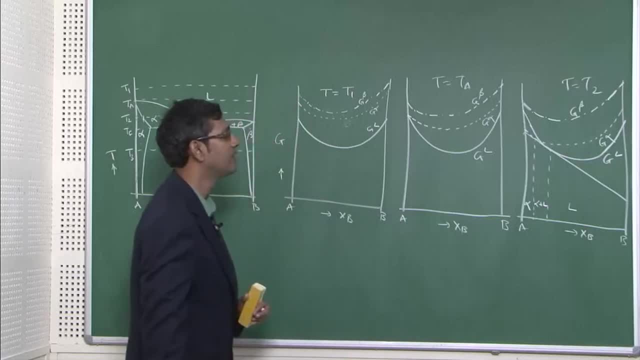 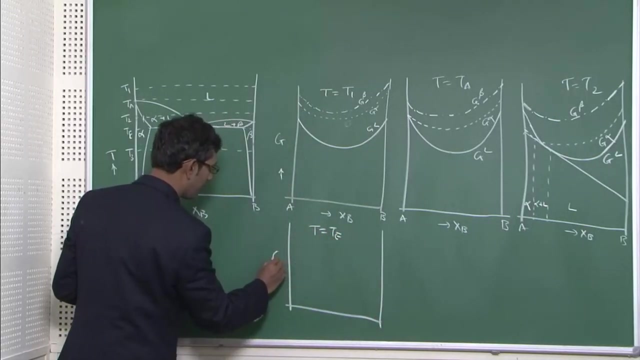 are potent. Both the pure A and pure B ends satisfy the things. So anyway, let us do at temperature equal to eutectic temperature, At eutectic temperature, at eutectic temperature. this is the classic temperature at which things 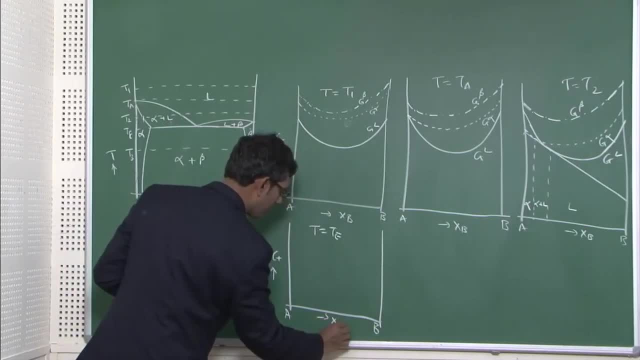 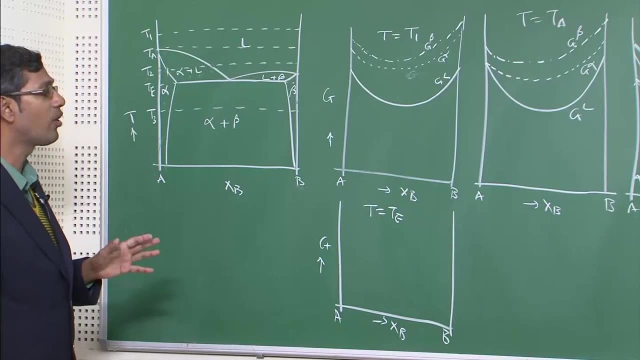 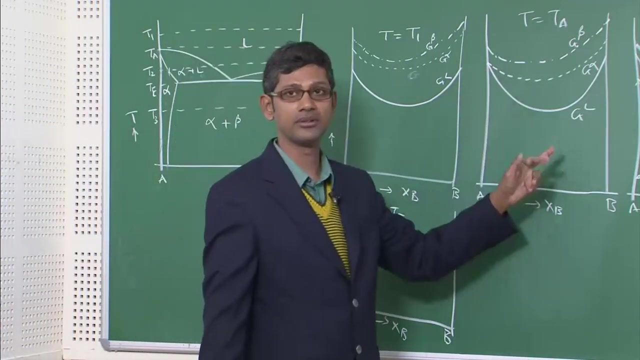 are different and distinct. What will happen At eutectic temperature? three phases- liquid and two solid phases- are in equilibrium, So that only is possible, Okay, Only when you have common tension between all the three curves done at a temperature. 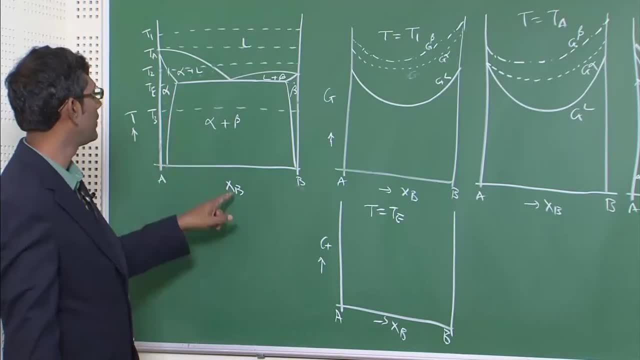 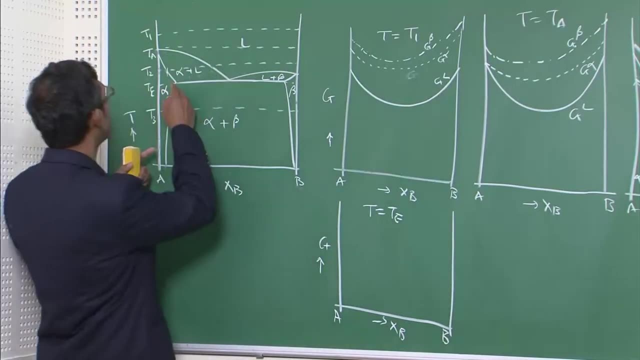 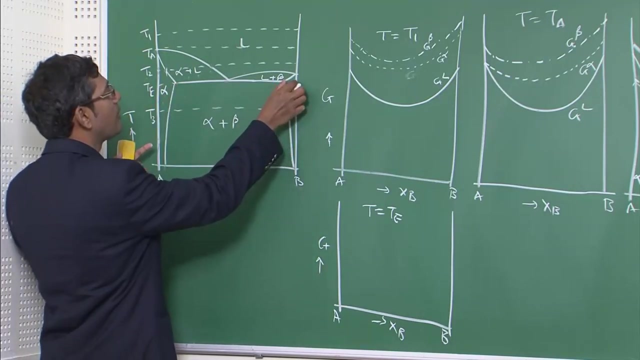 at a composition and equal to composition given by this phase diagram. So let us draw it. So let me first, because at your temperature you can see here, till this composition, this point: from this to this, the solid alpha is stable. from this to this, solid beta is stable. 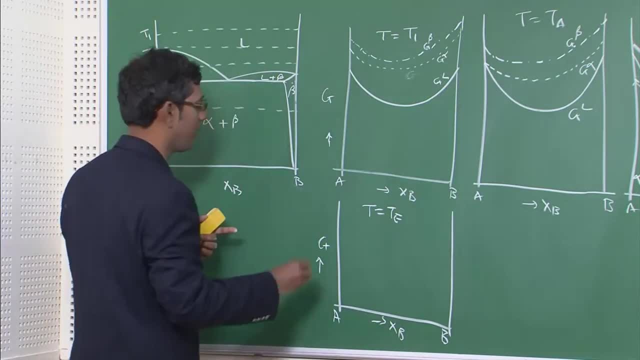 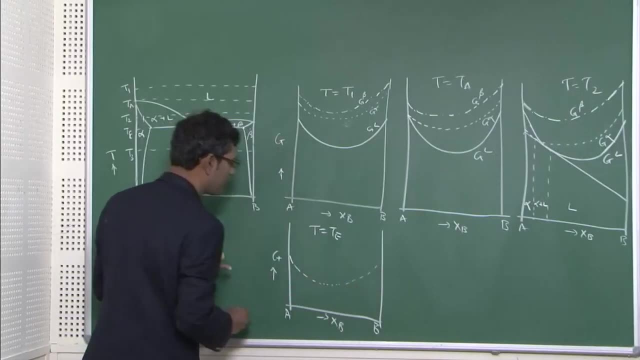 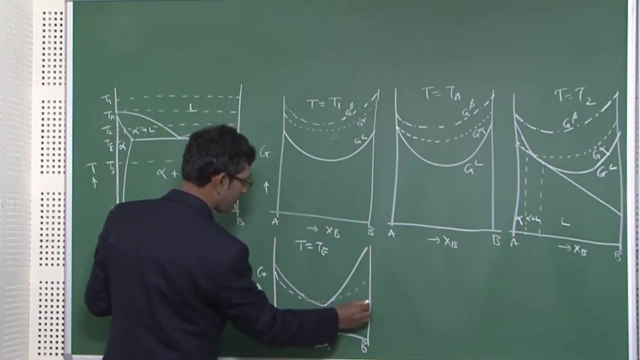 Only in this part. All these three phases are at equilibrium. So let me just draw solid alpha curve, Okay, and then I draw the liquid. cross over liquid will be like this. and then I draw the beta: Okay, Let me just put it. 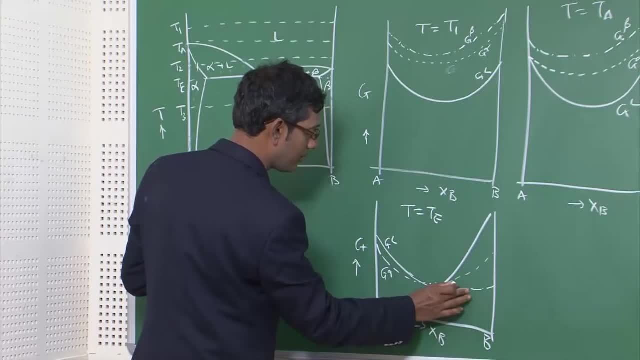 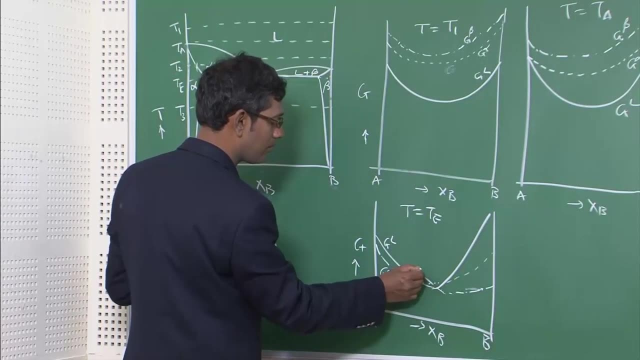 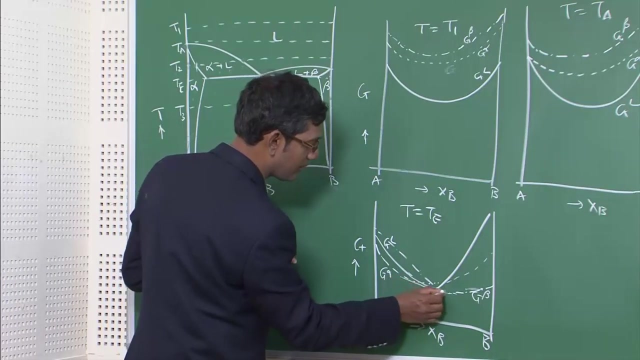 This is alpha, This is liquid. This is beta, This is beta. So you can clearly see, although I have not been able to do properly, these three curves are common, tangent each other. Okay, Okay, Okay, Okay, Okay. 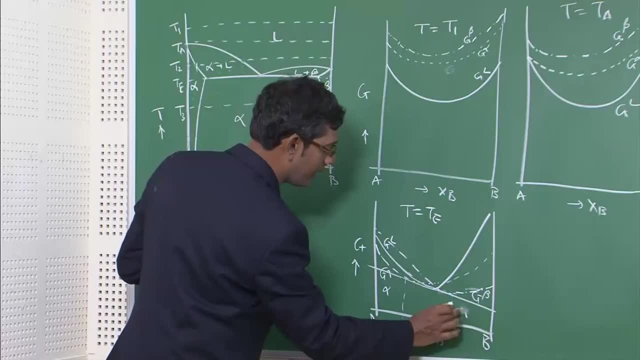 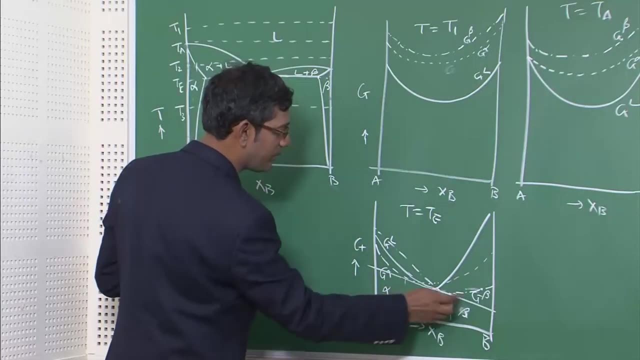 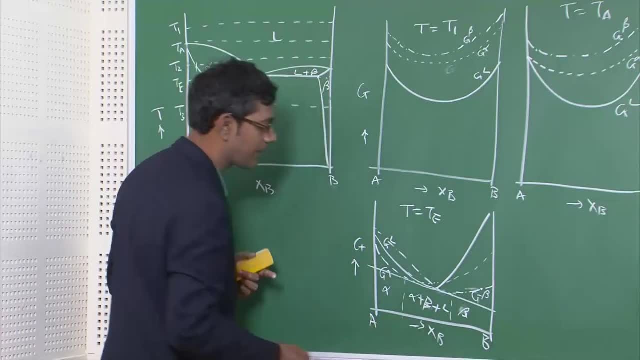 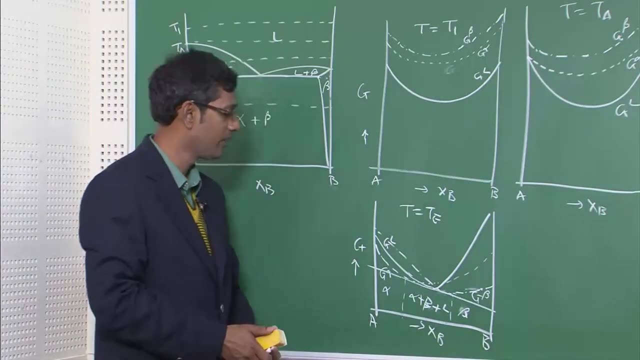 In between, three of them are at common tangent. So therefore, this will be the region of alpha plus beta plus liquid. Okay, That is what it is. Here, alpha, beta, liquid, three phases are coexisting. That is why, you can see, there is a composition domain. 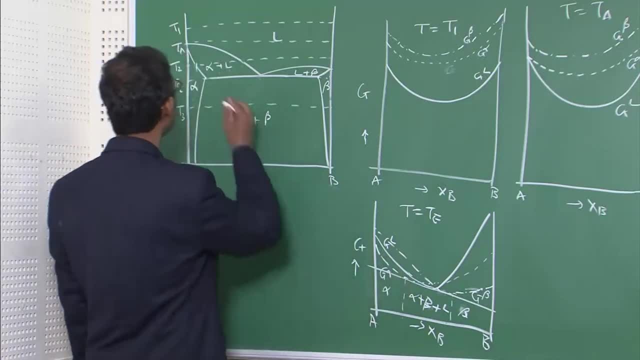 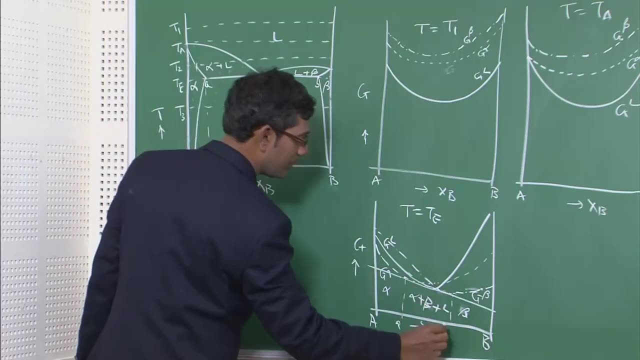 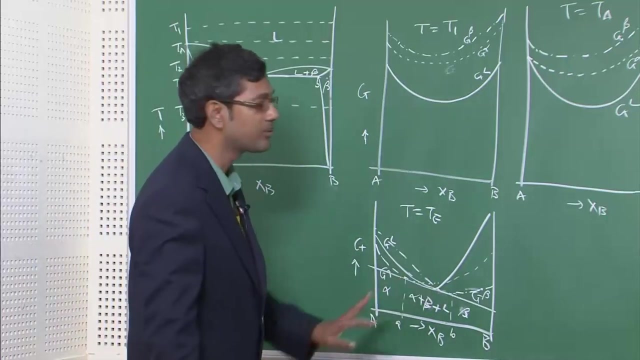 This is stable, Okay. point here I can mark at: A this is A. okay, A this is B. so this is P on the face diagram. That is how it is done. So therefore, at a temperature Te, all the 3 curves will be sitting. 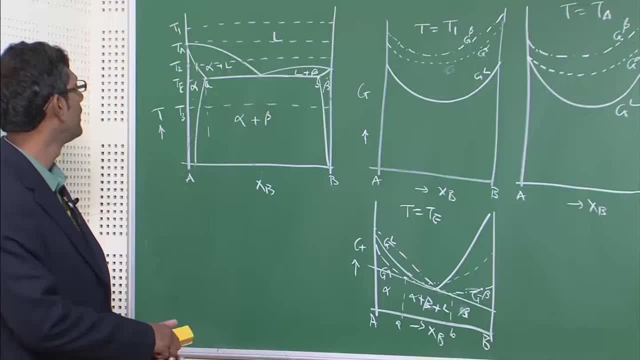 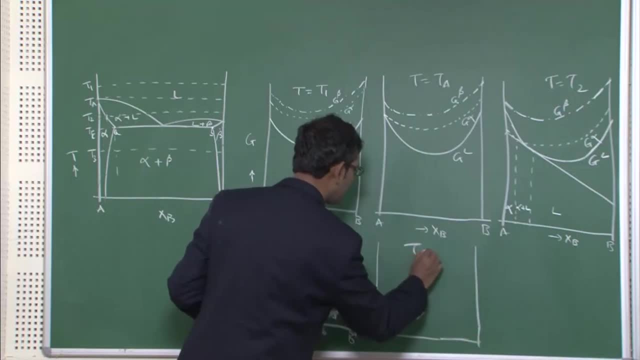 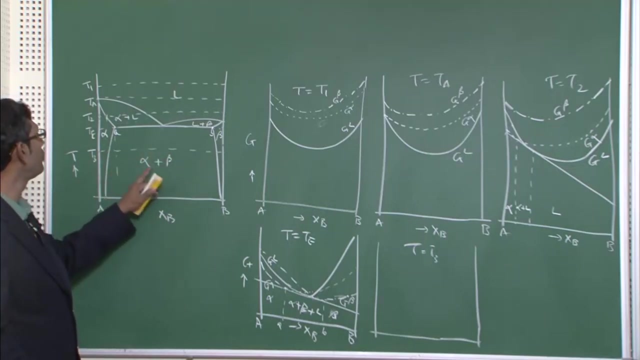 in such a way that you can draw a common tangent between them. So at T3 it is not difficult, much easy. At T3, liquid is not stable at all. at T3- it is at this temperature- only alpha and beta is stable. but there is a 2 phase field, alpha plus beta. therefore alpha and 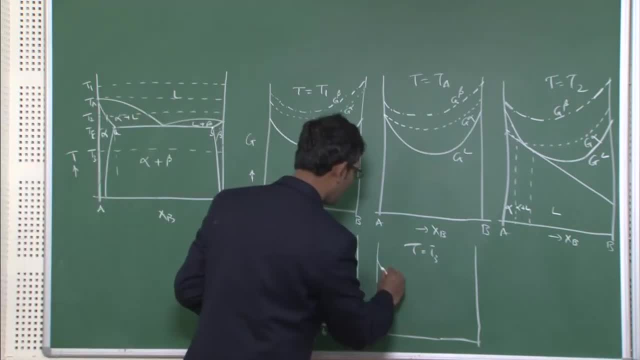 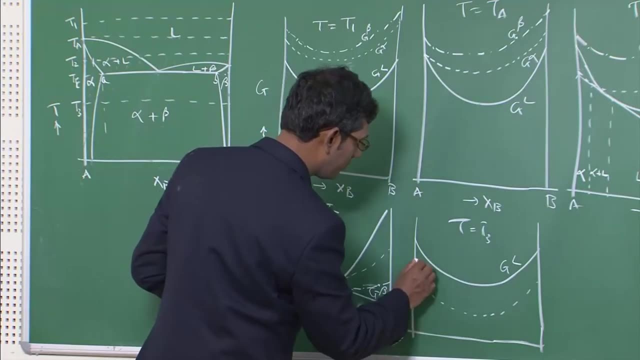 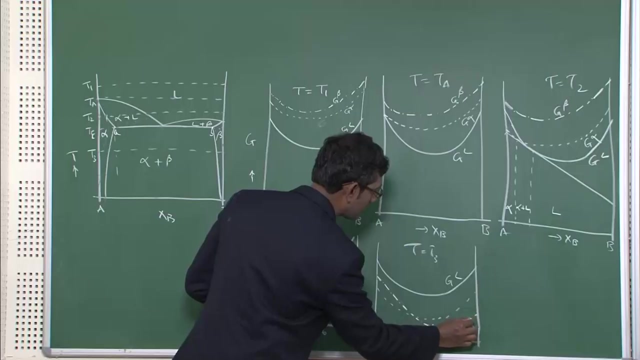 beta, the P and G curves will cross over, So liquid will be above G, L and alpha- okay. and then beta. beta is different, alpha is stable, Okay. So you can clearly see that alpha and beta are crossing over, so there is a common tangent. 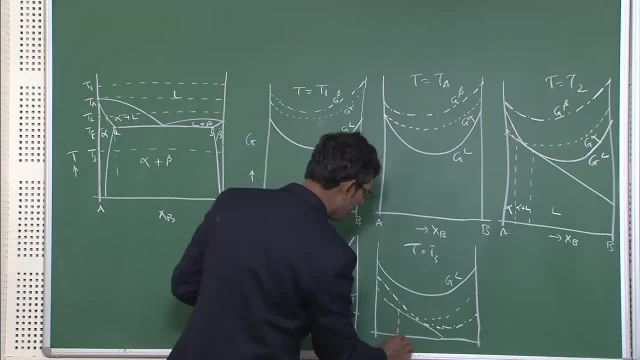 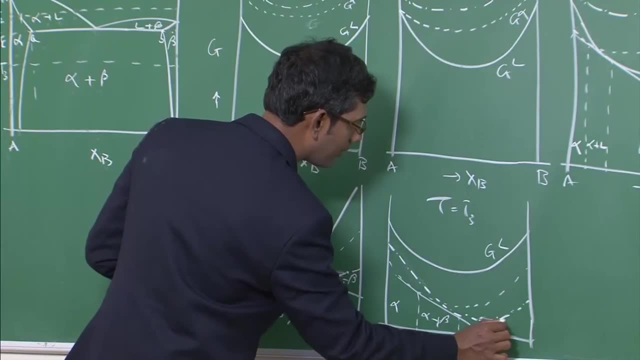 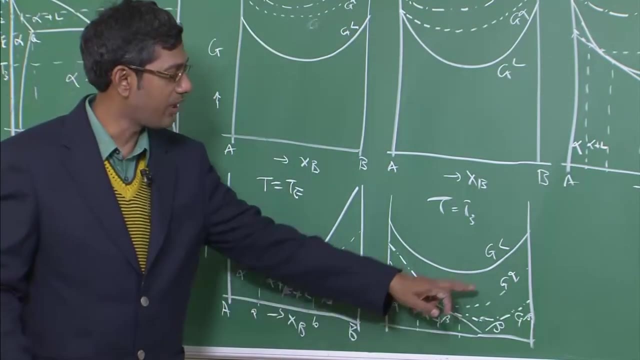 I can draw here between them. So this is what is, this is alpha, this is alpha plus beta and this is beta. Remember, this is G, beta, this is G, alpha, P and G curves. So you can always draw a common tangent between alpha and beta, P and G curves. 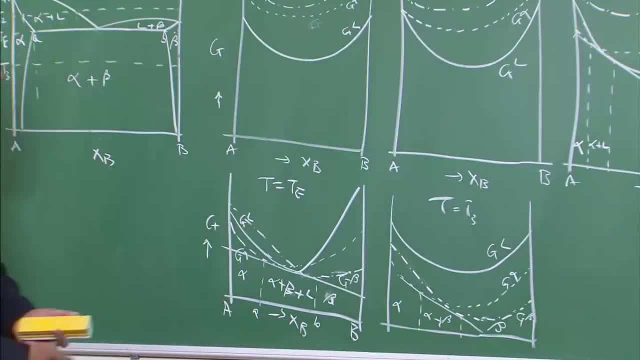 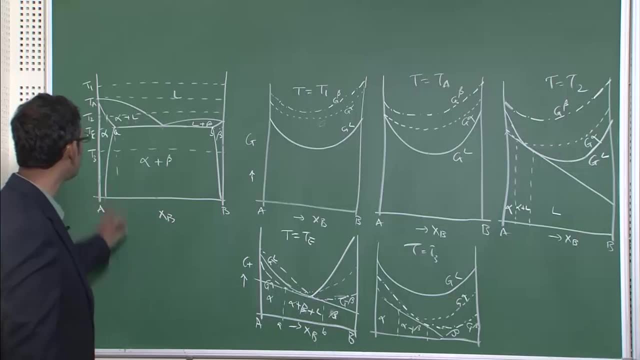 Okay, And then you can show that the common tangent actually demarcates the regions to be 2 phase region between the 2 single phase regions, alpha and beta. Okay, So that is how actually the P and G composition diagrams for the utility systems are drawn and I have shown you very. 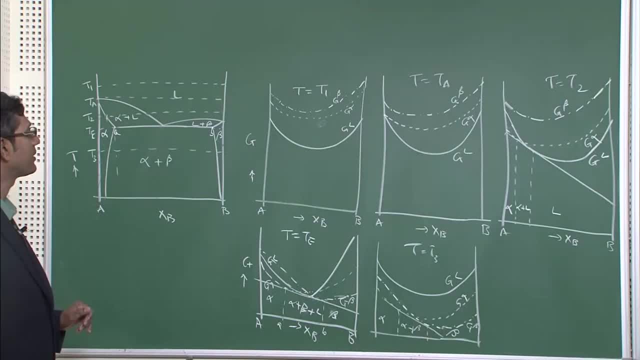 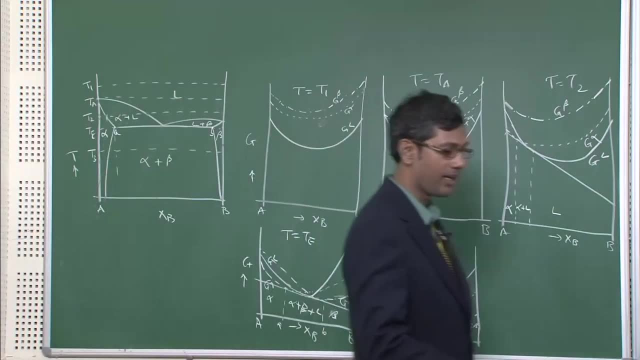 clearly that this is very important in the perspectives of understanding the phase diagrams, and you can do it for other systems also. So let me just go back, Thank you, And start discussing about aluminium silicon alloy. What will happen? And I told you that. 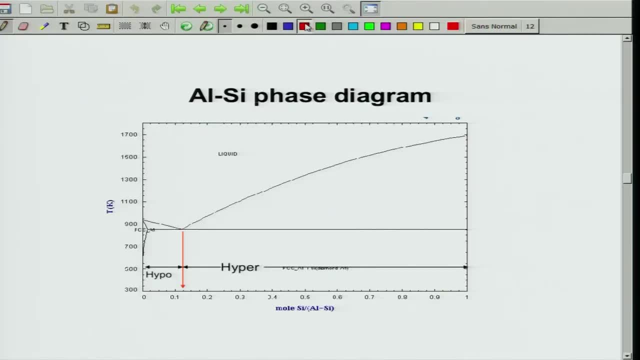 aluminium. silicon is a very important alloy system and this phase diagram is shown here. You can clearly see It is classical phase diagram in a sense that there is a uterative point here. a temperature and composition is given by this. It is about 11.8% of silicon. 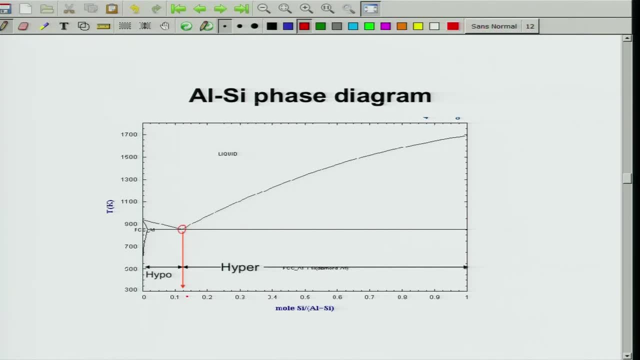 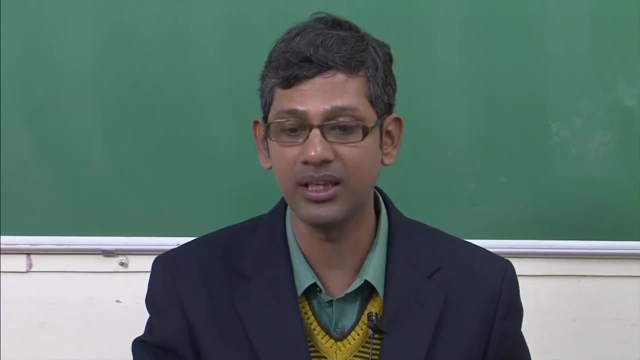 and temperature is about 573 degree Celsius. and, importantly, you have a single phase zone here, alpha, which is solution of silicon and aluminium, but on the right side, silicon inside, there is no such thing, it is a pure silicon. So now I know that the alloys which are important for industrial applications are the hypo-eutectic. 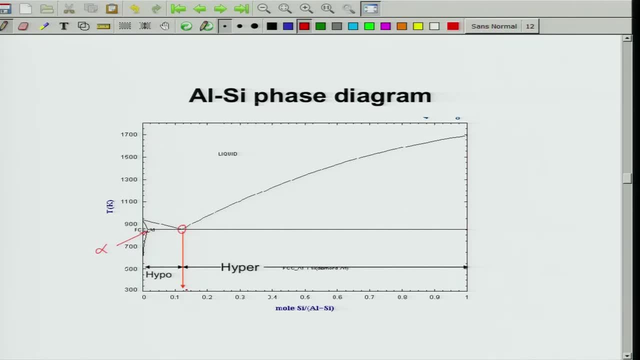 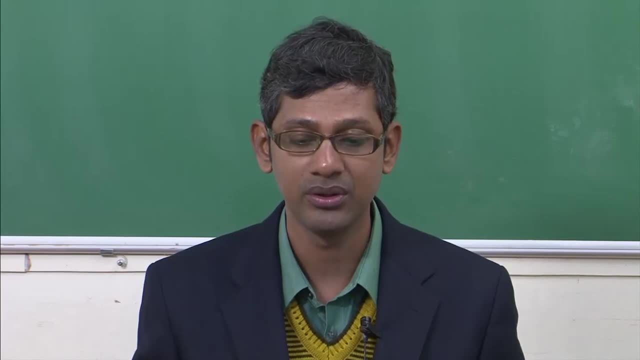 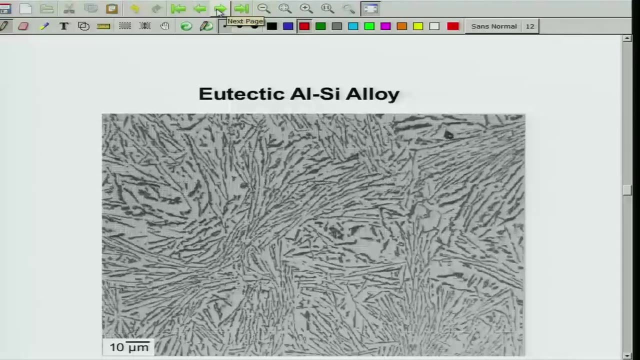 alloys. alloys which has compositions less than eutectic hyper ones are not very interesting because it contains hard silicon particles. that makes the alloy very brittle, not used. So the next slide, this is the classical aluminium silicon alloy microstructure I have shown. 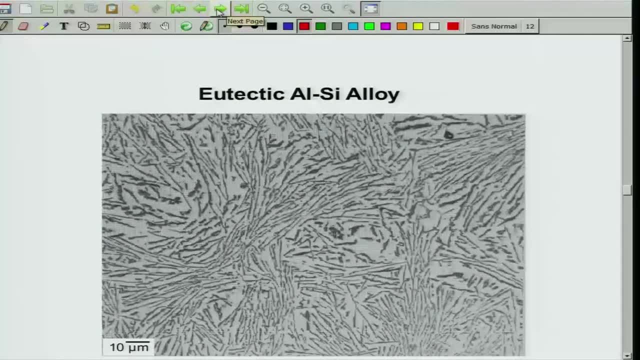 you already, it contains continuous white aluminium matrix like thing, but it is not a matrix, it is basically aluminium phase. and then you have needle like silicon. Now, as I told you, silicon is very brittle. if I take a silicon piece and just drop it on the floor, it will break or shatter into pieces. 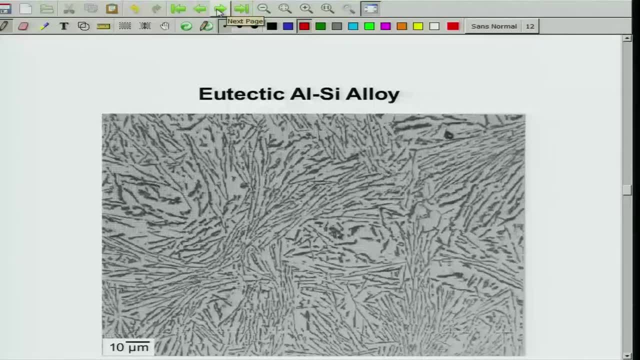 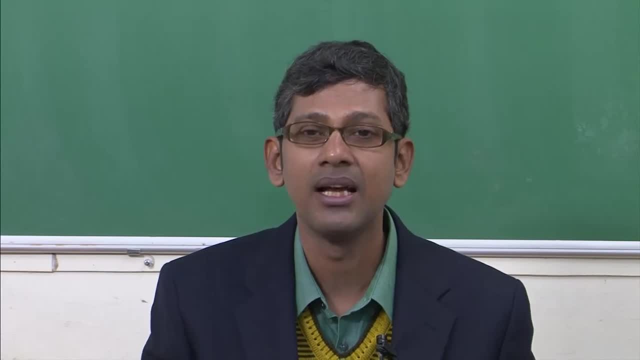 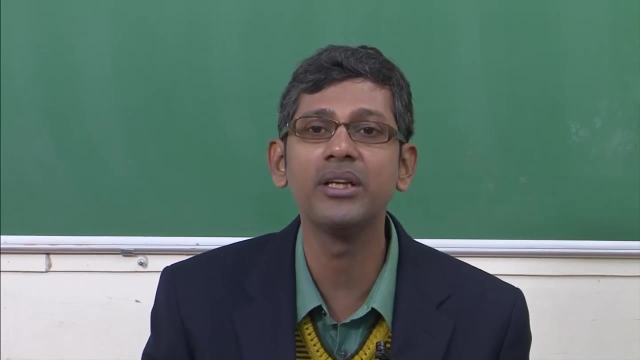 And so, therefore, these needles are basically makes the alloy brittle not so good. So we need to modify this microstructure, and this is very important in the sense that you need good machinability, good toughness and ductility of the alloy when you are using. 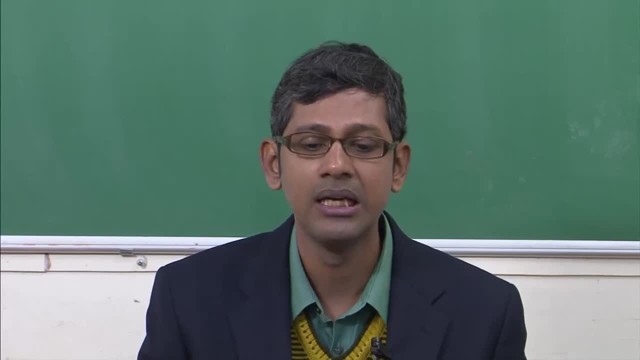 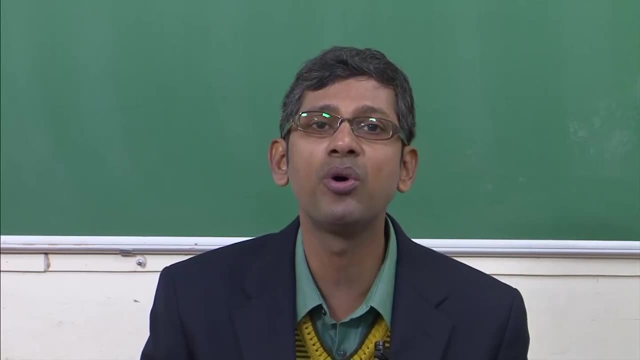 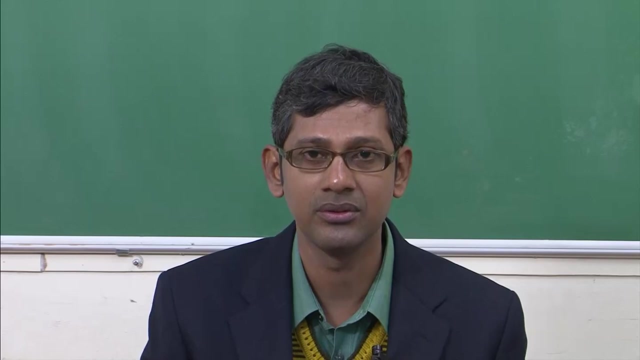 it as an engine block for many of the car engines. So what is done- and this is serendipity in the metallurgy or materials engineering- is that you add very small amount of sodium, Sodium or arath, and amount is very small. it is about 0.1 percentage. 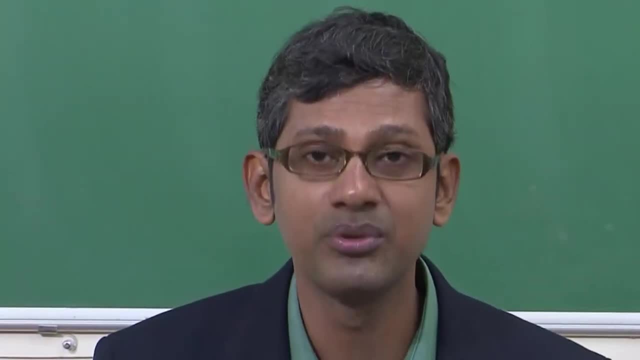 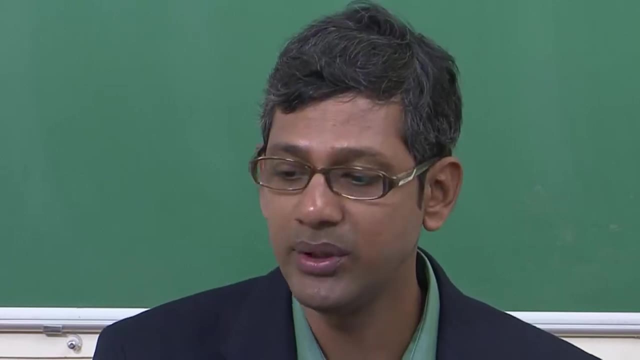 So that means if you use about 100 grams of the aluminium silicon alloy, you need about 0.1 gram of sodium or strontium. Sodium is Na, strontium is Sr or rare earth metals or mixture of rare earth metals sometime. 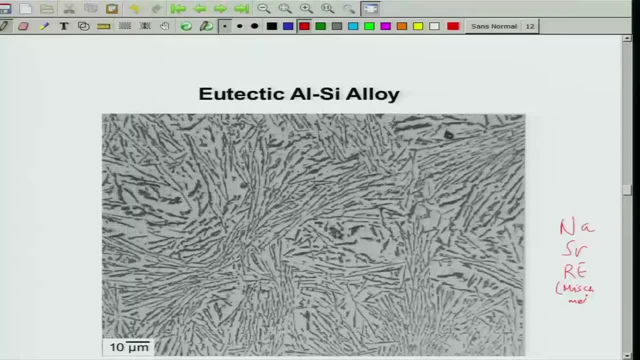 it is known as MISCH metal M-I-S-C-H. MISCH metal 1, 2, 3, 4.. 1, 2, 3, 4.. 1, 2, 3.. 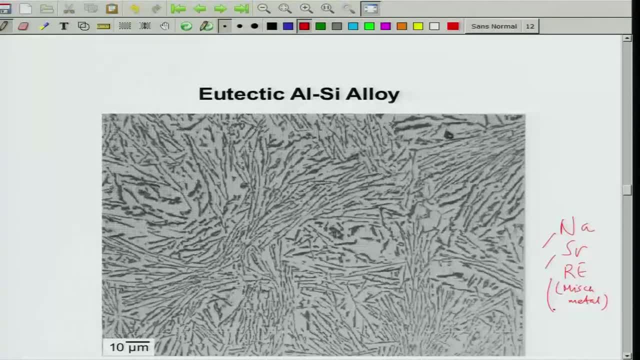 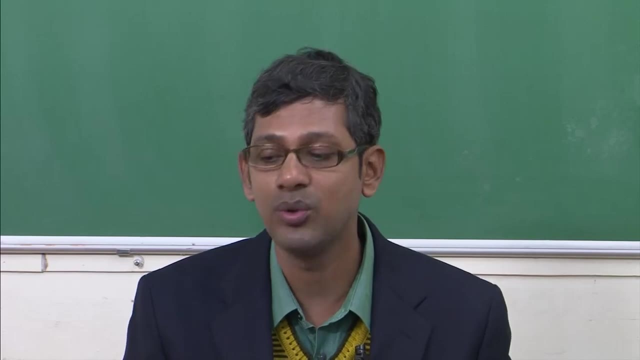 3 different types of things are added, sometime together, sometime separately, to modify the microstructure, to modify the silicon needles, and this has been discovered out of serendipity. Nobody knew that it will happen. Somebody probably had tried to add sodium into it and then found that microstructure. 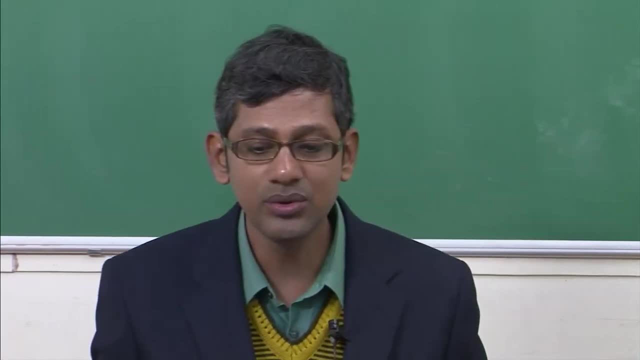 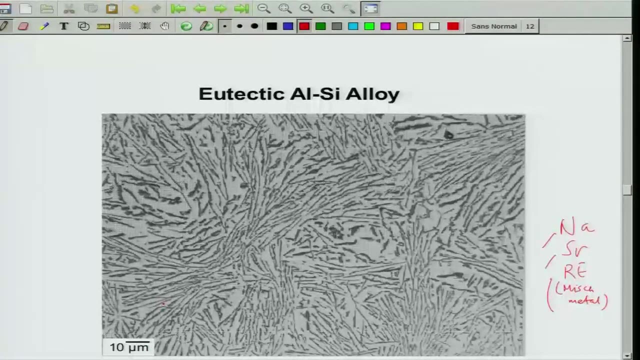 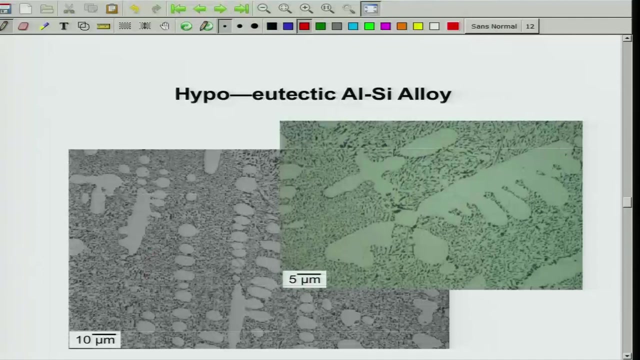 do get changed. What is the change you see? Change you see is this: you can clearly see the earlier picture. this is 10 micrometer scale. The silicon needles are very big and quite thick also. On the other hand, if you add about 0.1% silicon, the silicon needles become very fine, very 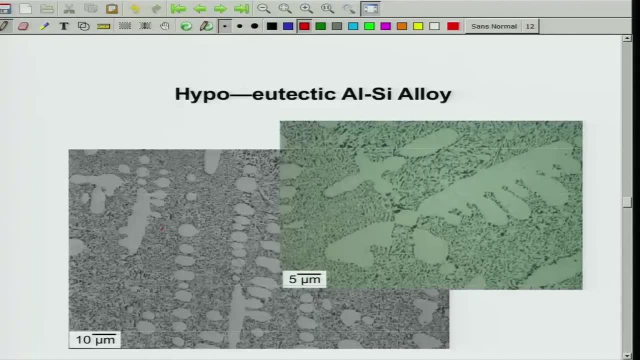 very fine silicon needles become. Not only that, you also find some amount of aluminium which is alpha aluminium, which is present in the microstructure. It is shown at a high magnification view here you can see the micron bar is 5 micron now. 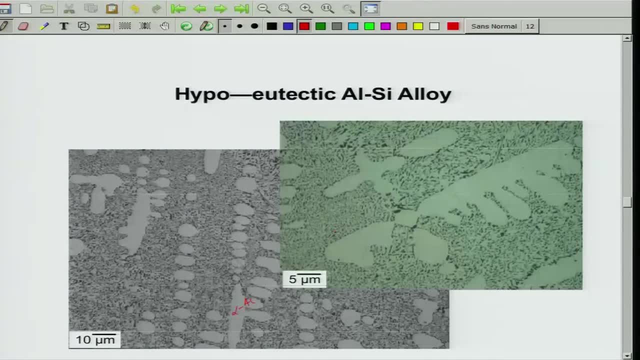 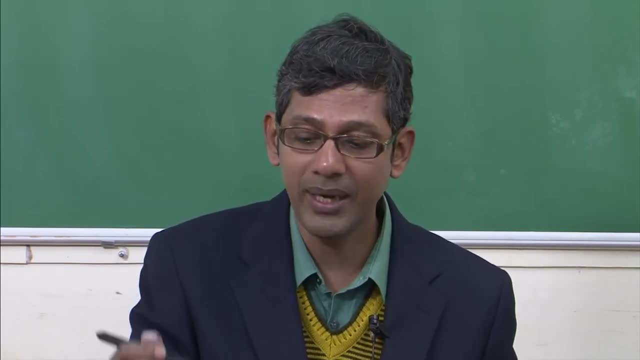 So you can modify the silicon needles or eutectic, rather Very little, Very little, But you can make it fine scale and, as you know, if you make something by this finer scale, your ductility and strength both improves. So by making this as finer, we improve the ductility, we improve the toughness. 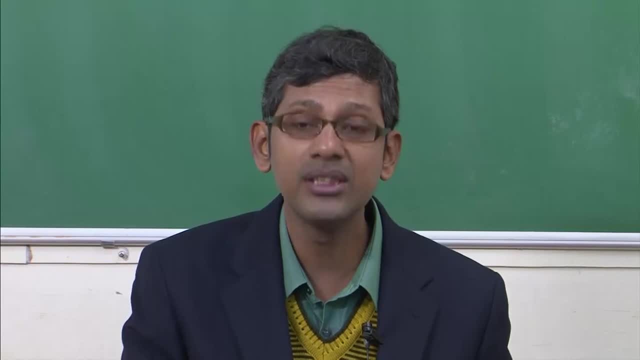 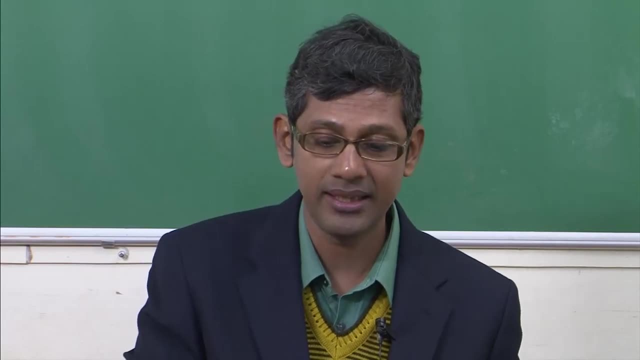 At the same time, we do not change the strength much. So this is what you want, This is what industry people want. They want a wonderful material which will be used for many applications, and that is what you see here. But you know, the important part is this: 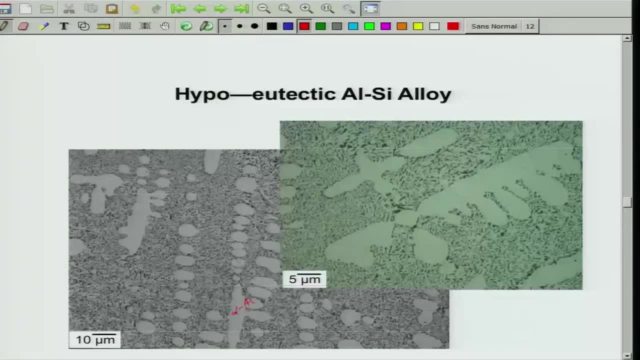 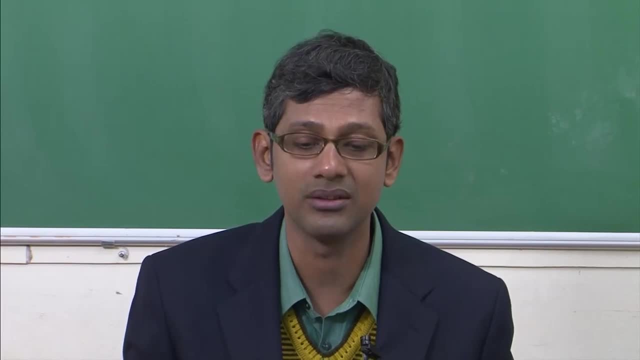 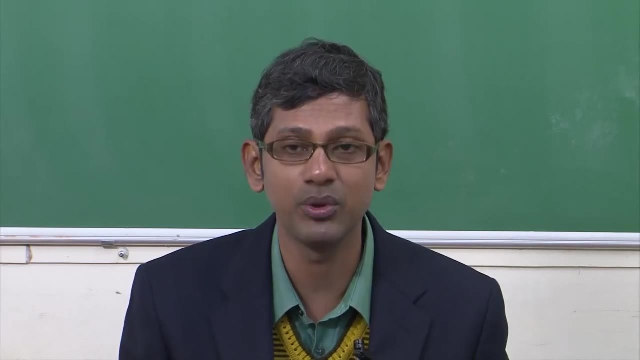 In all this microstructure you see presence of alpha aluminium dendrites. So that means what That means: this alloy is not behaving like eutectic alloy, it has become a hypo eutectic alloy. So this particular phenomenon of modifying this eutectic microstructure modification 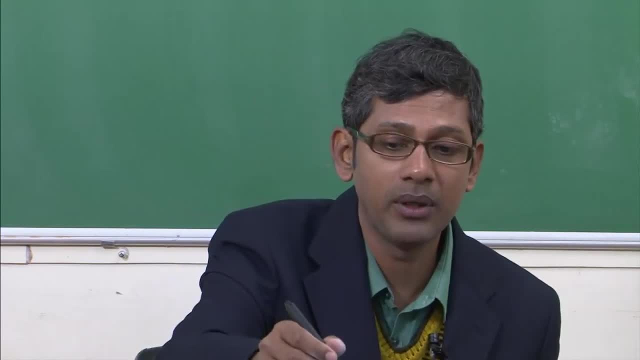 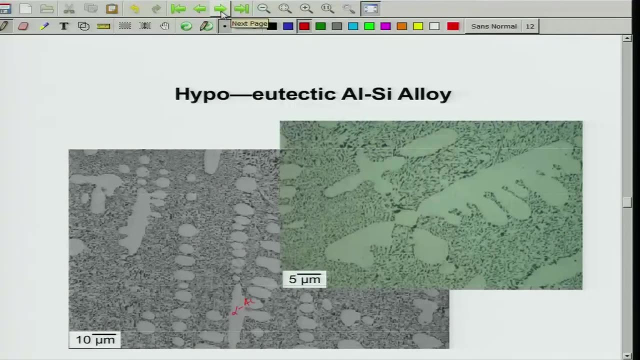 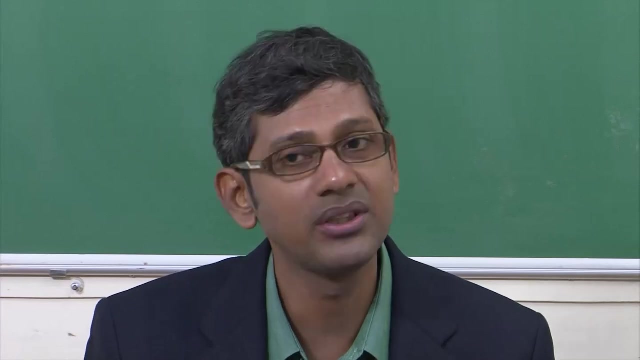 of eutectic microstructure from a course of this microstructure like this to a fine ones like this is known as modification in the literature and this is routinely done in industry nowadays and this can be explained using free energy composition diagram again, but I will not go into that details. but let me tell you what actually happens. 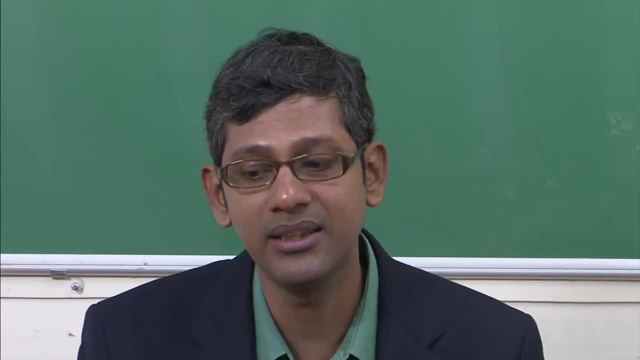 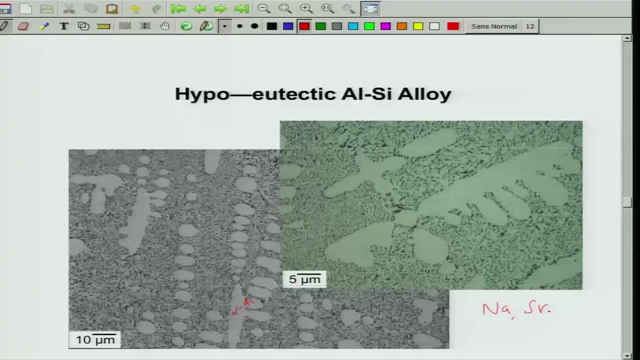 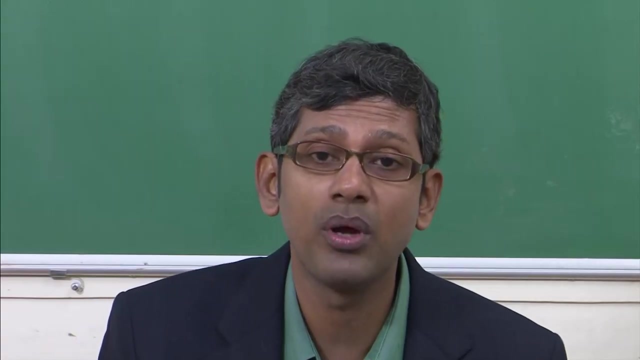 If you add sodium or if you add some amount of strontium or whatever it is sodium, strontium or any mis-metal or error metals like that- they actually hinder the growth of silicon metals. Remember, silicon is a metalloid. it has its own growth problems. 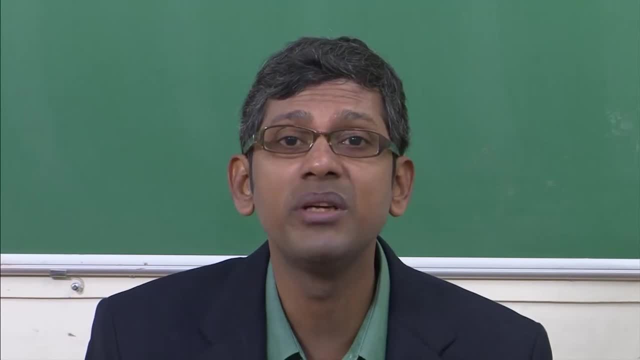 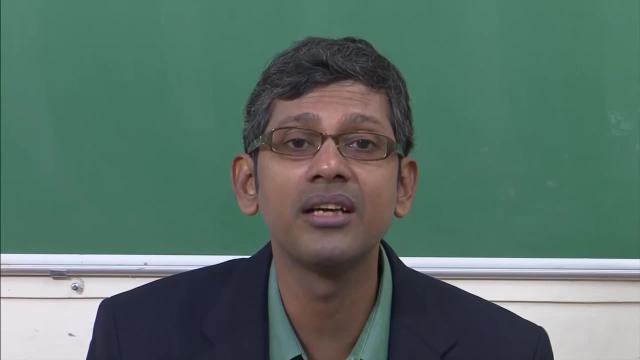 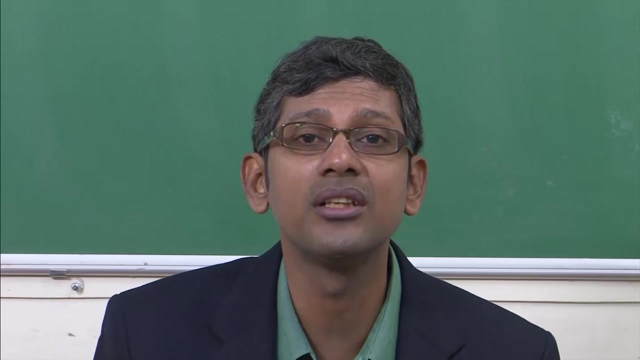 Unlike other metals, like aluminum copper, It cannot grow very nicely. it cannot grow nicely in the sense that when atoms actually jump and sit on the surfaces of silicon, they cannot get attached along any plane. they need to be attached along certain twin boundaries and I am not going to get details into those. 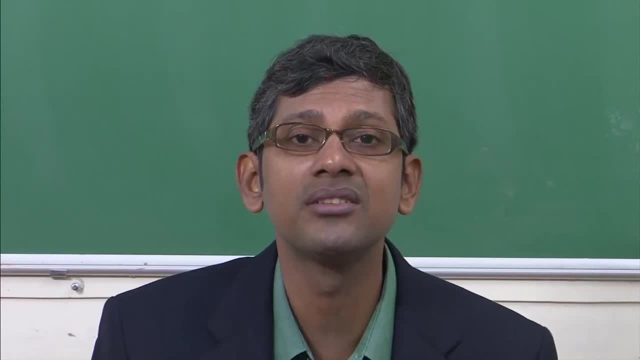 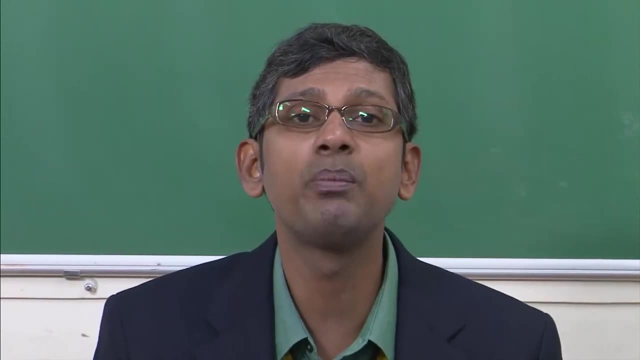 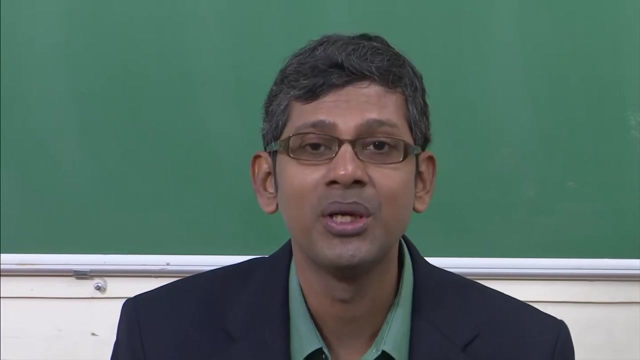 because those are will lead to, you know, different discussions deviating from the actual syllabus of the course, but you can read. these are very interesting. So sodium actually poisons The growth of silicon needles. Sodium sits on the silicon needle and it has been observed that it poisons. Basically it does not poisons that. it removes the phosphorus: Sodium, strontium, whatever is the elements they scavenge out the phosphorus in the melt. and if they scavenge out the phosphorus in the melt, silicon cannot nucleate very easily. 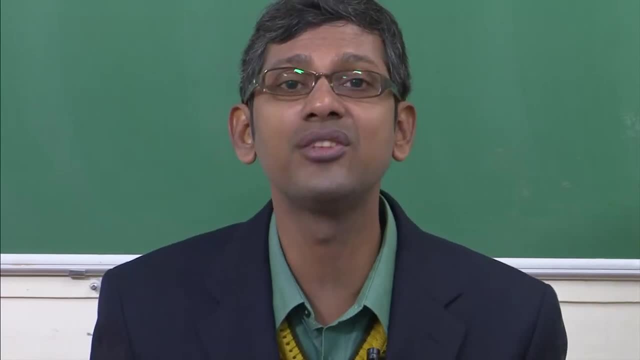 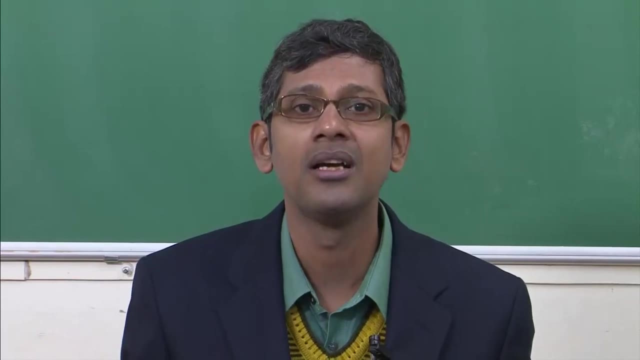 So what is the scavenging out? What actually happens is that if I add sodium, strontium or some mis-metal into the melt, react to the phosphorus in the melt. What happens? The phosphorus in the liquid which is present, and you may be thinking where from the phosphorus? 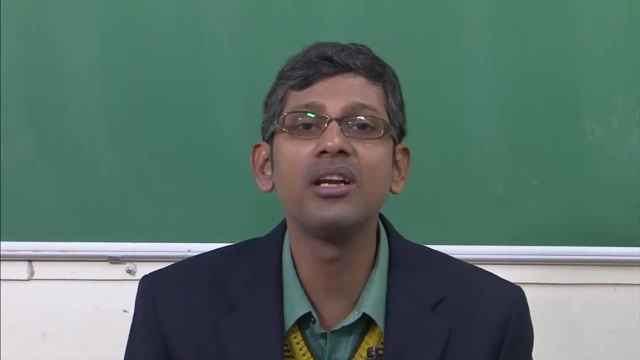 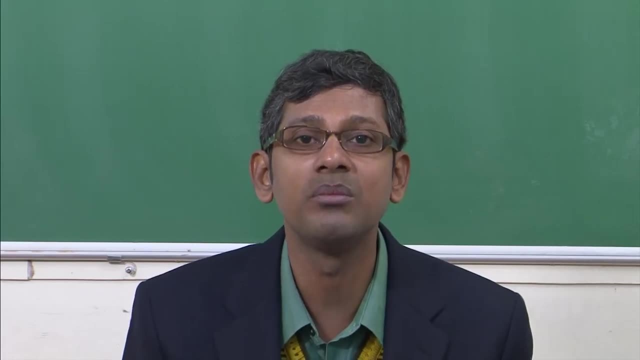 come. Okay, that is a very good question. Phosphorus actually comes from the liquid itself, from the ore: Aluminum, silicon alloys- whenever prepared, we add the commercial purity aluminum and commercial purity aluminum will have lot of phosphorus into it and this phosphorus actually 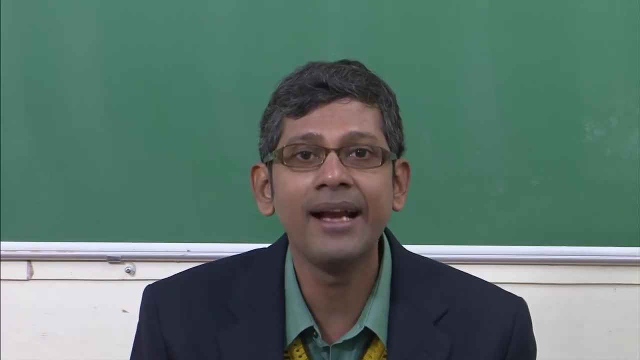 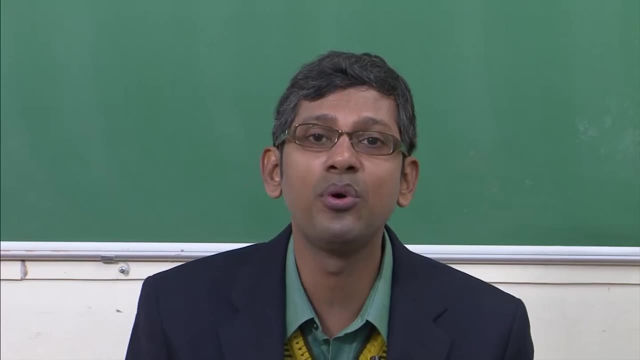 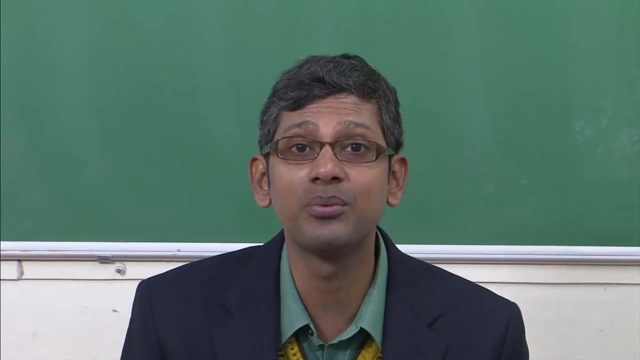 form react to the aluminum, from aluminum phosphide and on the aluminum phosphide silicon needles they nucleate and grow and become very long. So therefore, if I add sodium or if I add strontium and this sodium and strontium preferentially react to this phosphorus and remove the phosphorus from the liquid so that aluminum phosphide. 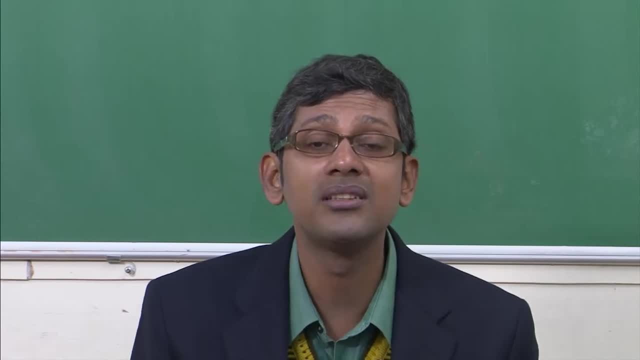 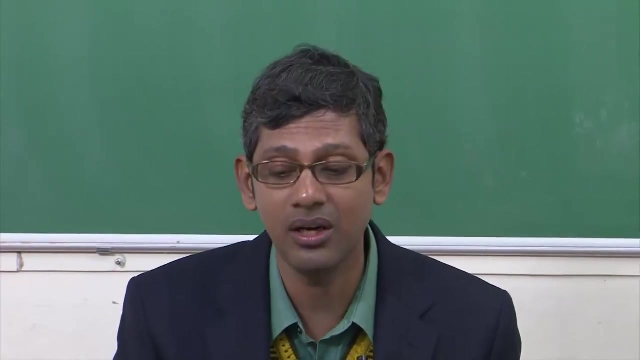 cannot form. If the aluminum phosphide cannot form, silicon cannot nucleate on aluminum phosphide. So therefore the nucleus of silicon is prolongated and this lead to very finer silicon needles in the microstructure. That is what you see: a very fine scale silicon needles, very fine scale structure. 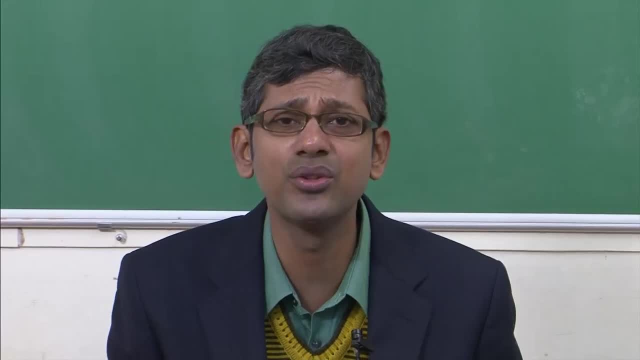 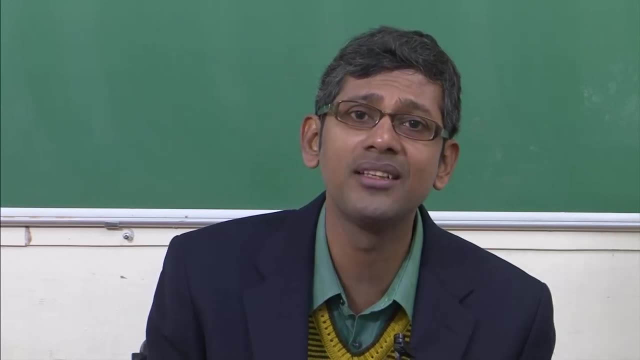 So that is how things happens. There are other theories also. In fact, to be frank, this is not completely understood in materials and metallurgical engineering how actually things happen. The other theory is that in commercial purity aluminum you can have iron as on the impurity. in aluminum alloys and iron. with aluminum and silicon can form iron aluminides, iron silicides, actually A L F E S I type of phase. and this A L F E S I type of phase then can prolongate, or rather make the nucleation of silicon difficult, and that is why silicon become finer. Anyway, let us forget about iron, but let us only think about that. in aluminum silicon alloy your phosphorus present and this phosphorus reacts with aluminum and from aluminum phosphide, and this aluminum phosphide helps in nucleation of silicon. that is why you have easy nucleation. of silicon. That is why it grows very fast. but whenever you add sodium or froncium or other metals, it reacts with phosphorus, removes the phosphorus from the melt so that aluminum phosphide cannot be formed and because of the silicon, nucleation is difficult. I mean silicon is very difficult. 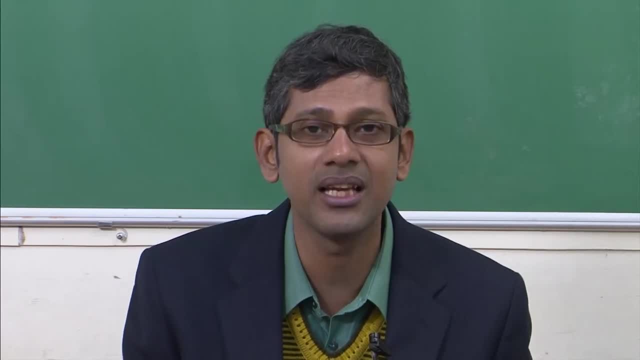 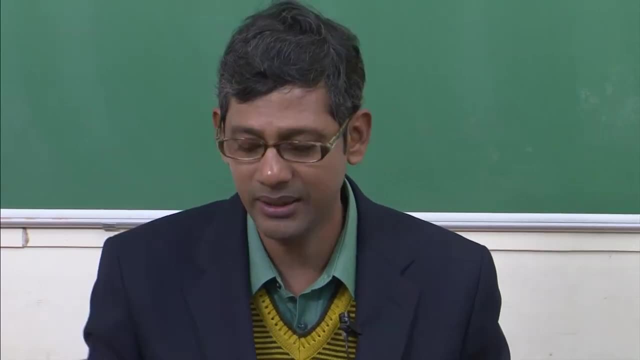 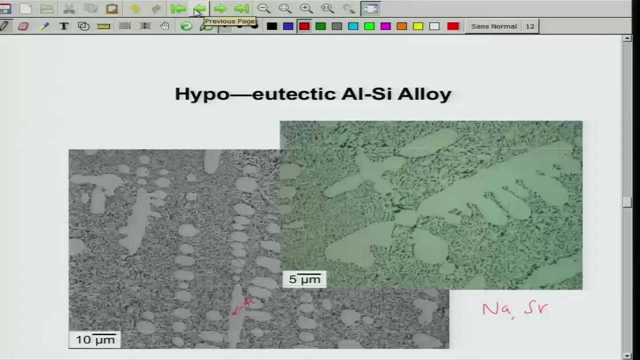 to nucleate, then it will not grow large. it remain finer scale and that is how thing happens. This can be explained very easily using the phase diagram data. Let me just go back. Let me see whether I have in here. Okay, So let me just go back and explain it using the phase diagram. 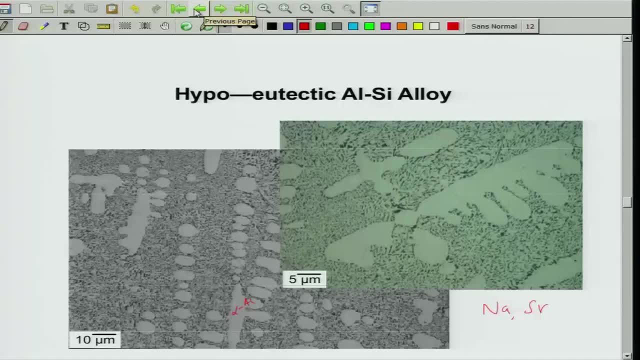 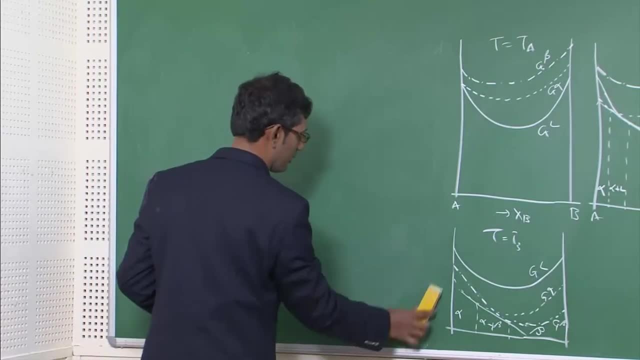 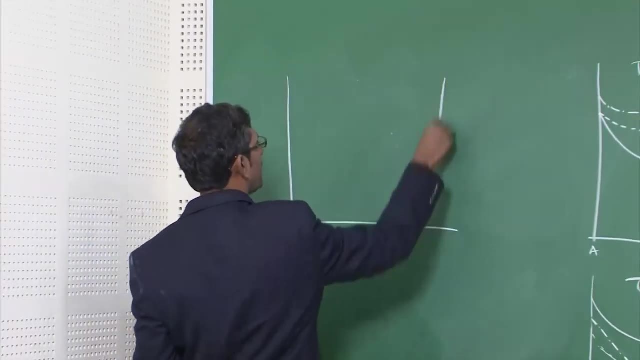 So what does it mean is that if I have a problem in nucleation of silicon in the liquid, so what it will do? It will basically lead to more under cooling. So that means if I have a aluminum silicon phase diagram like this, this is aluminum. 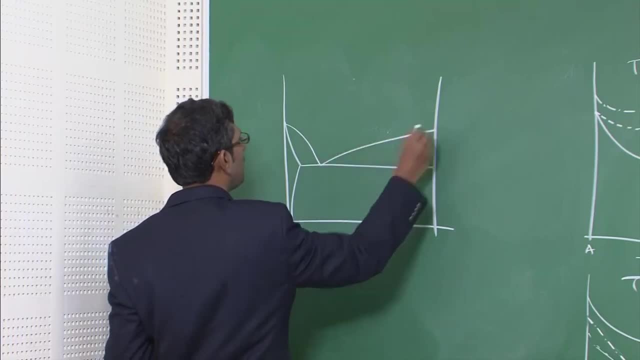 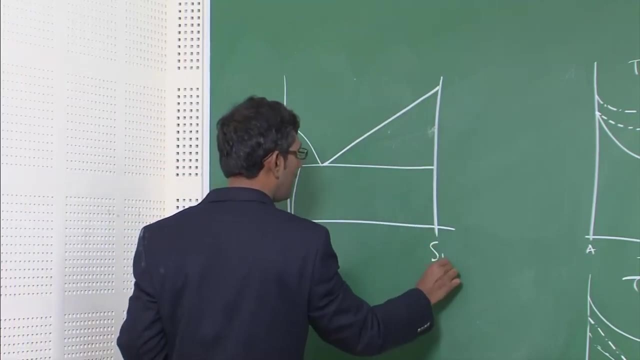 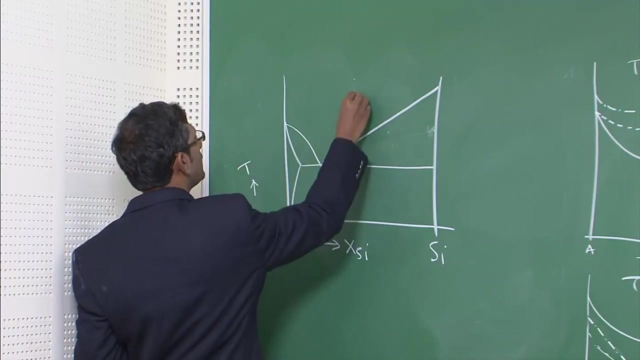 silicon pure. Correct, Sorry, Okay, This will be up. Okay, This is silicon has a much higher melting temperature. So this is silicon. this is XSI, or mole fraction of silicon. this is aluminum. this is temperature. this is liquid. this is alpha aluminum plus silicon. this is liquid plus silicon. this 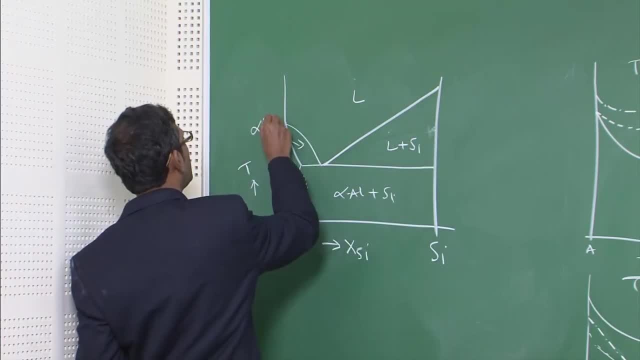 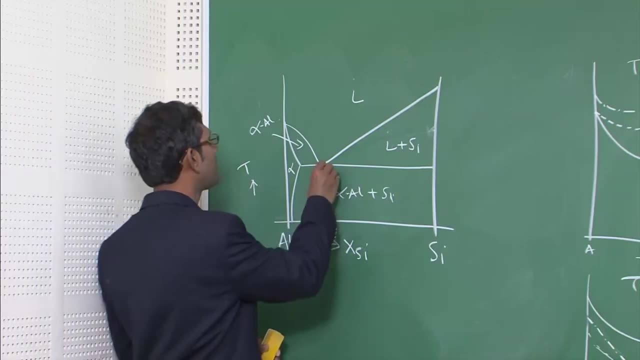 is alpha aluminum, and this will be alpha aluminum phase diagram. This is what is the phase diagram looks like Now, the moment you add silicon, and this composition actually sits at 11.5.. Okay, This is the phase diagram. Silicon actually sits at 11.8.. 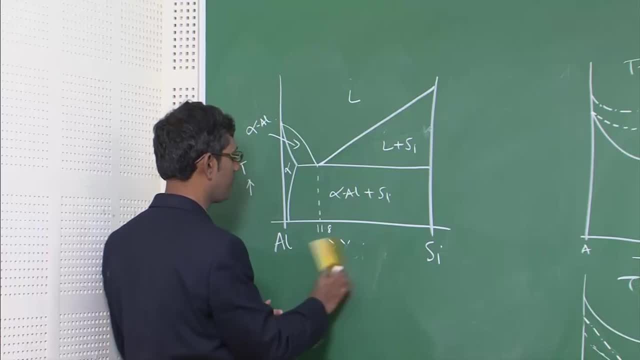 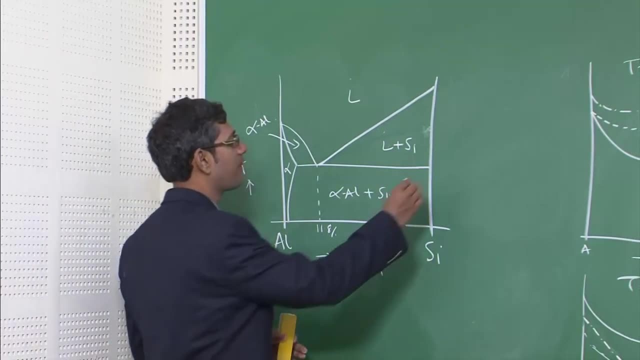 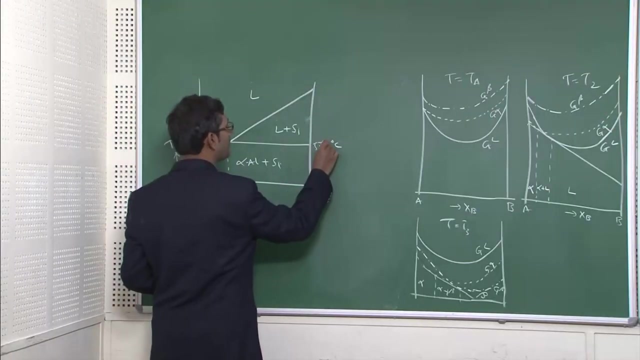 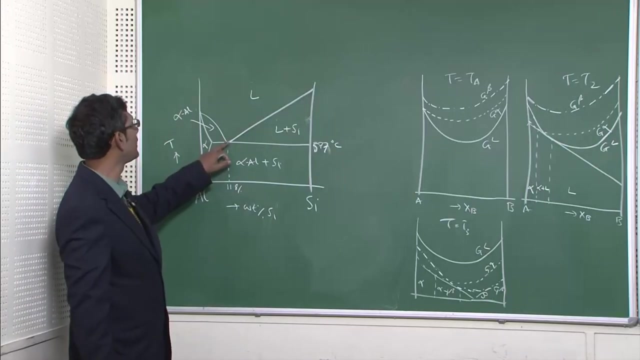 Okay, Remove this. let us write: weight percent of silicon: 11.8 weight percent of silicon and this temperature is something like 573 degree Celsius. Okay, Sorry, 577 degree Celsius, not 73.. I hope you can see it carefully: 577 degree Celsius. 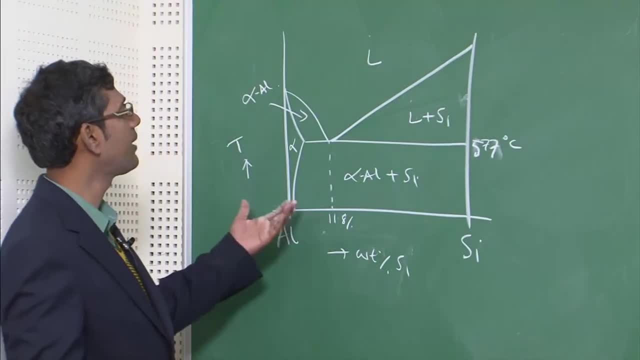 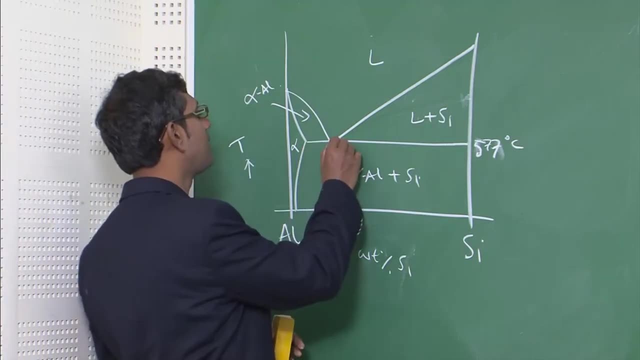 This is the eutectic temperature, eutectic composition. Okay, So whenever I add sodium or strontium or some other metals to modify it, what does it mean is that the eutectic temperature and composition shifts to higher? 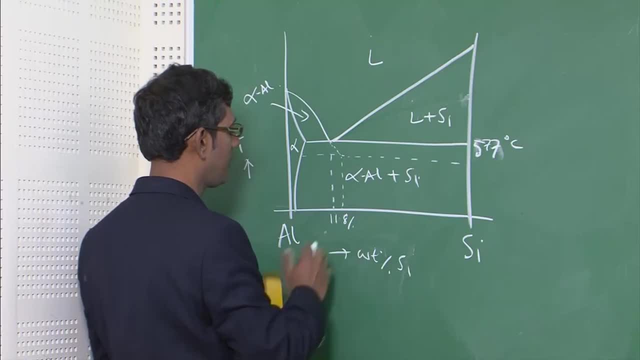 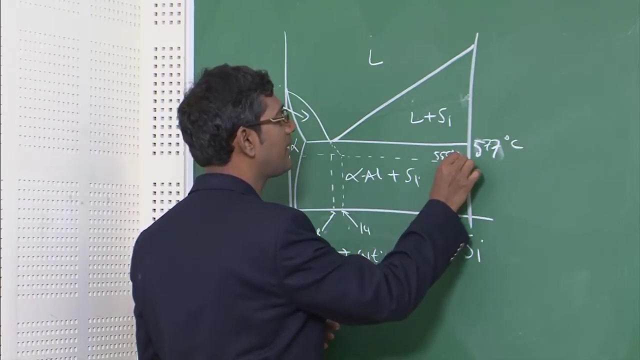 Composition shifts to higher, it becomes actually 14%. So this is 11, original one 11.8 and this one is 14 weight percent and this temperature is 555 degree Celsius. Okay, So that means what? If you make this silicon nucleation difficult, it requires further 22 degrees of. Difference between 577 and 555 is 22 degrees, So this leads to change the eutectic composition to 14 atom percent. So therefore the eutectic alloy, which was originally eutectic alloy, now has become a hypo-eutectic alloy. 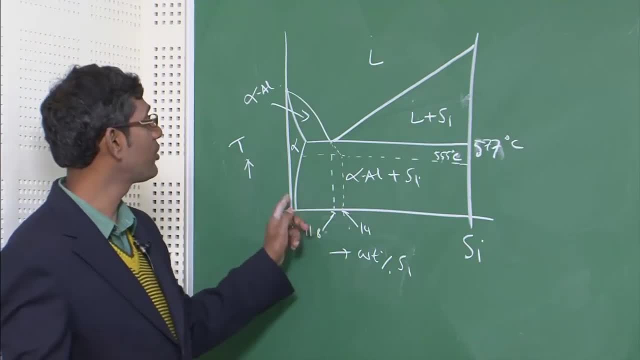 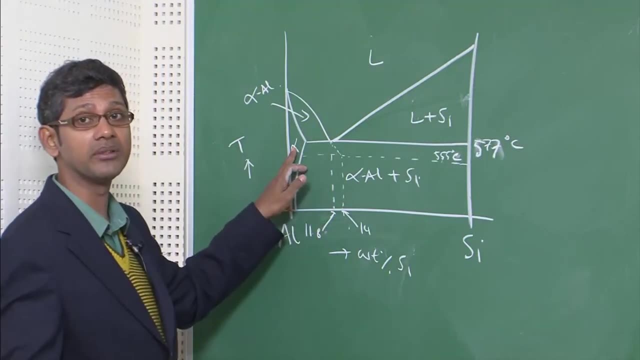 Is it clear. It becomes a hypo-eutectic alloy and because of this hypo-eutectic nature, it is in the form of alpha-aluminium dendrites in the liquid. That is why you see alpha-aluminium dendrites in the microstructure which I have shown you. 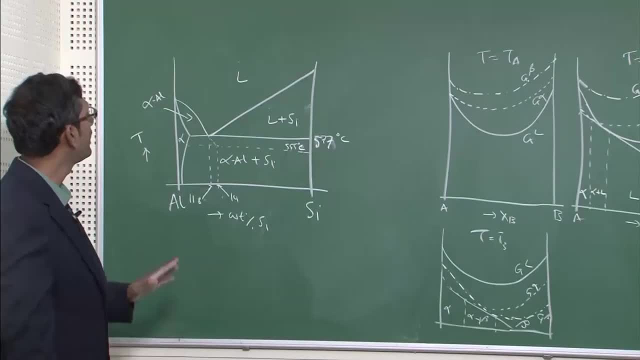 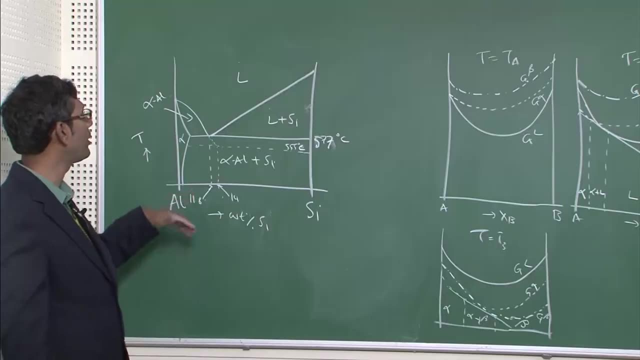 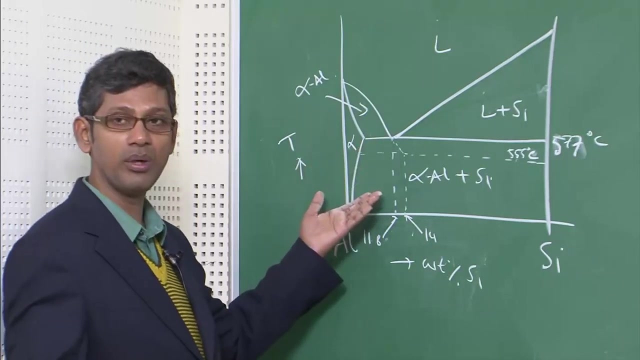 So basically what it boils down is that, in a short way, that if you add sodium, strontium or something, it basically makes the growth or nucleation and growth of silicon difficult. Basically, growth of silicon makes it difficult and that is why you need more under cooling. 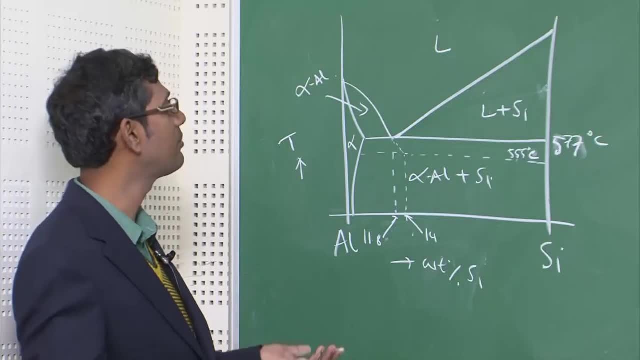 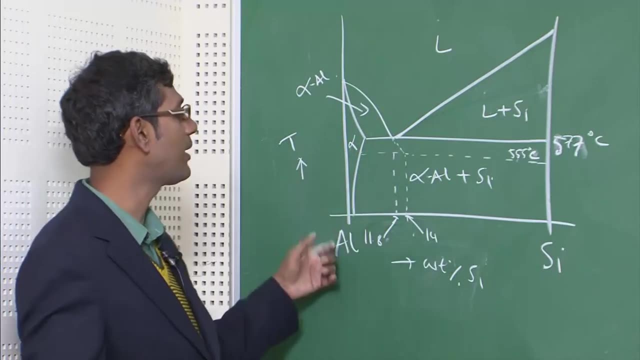 because you need to provide more- Okay, More- energy to the system, and then it has become a hypo. you know, the same alloy which was eutectic alloy for aluminum silicon. when you add sodium, it becomes hypo-eutectic alloy. 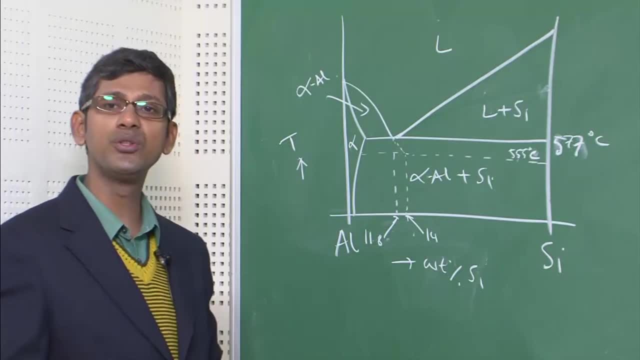 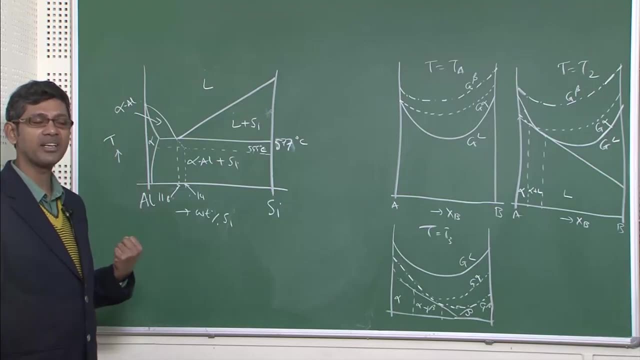 and you get to see some lot of aluminum dendrites and, as you know, aluminum is actually very soft metal. So therefore, aluminum dendrites will make this alloy soft, tactile and tough At the same time as the eutectic has become finer. it will also lead to high strength.